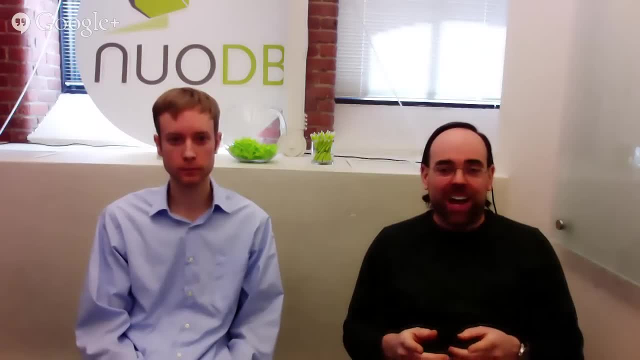 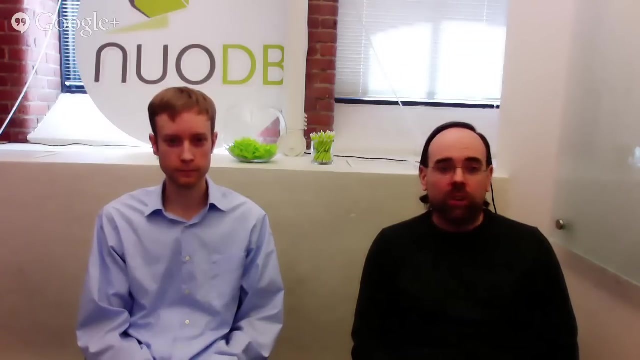 I do want to say, for those of you who missed it, it's been a pretty awesome week here at NuoDB HQ here in fabulous Cambridge Massachusetts. Yesterday we announced another round of funding, which we're pretty excited about, And a round led by a really really big, really awesome customer of ours, Daso C-STEM. 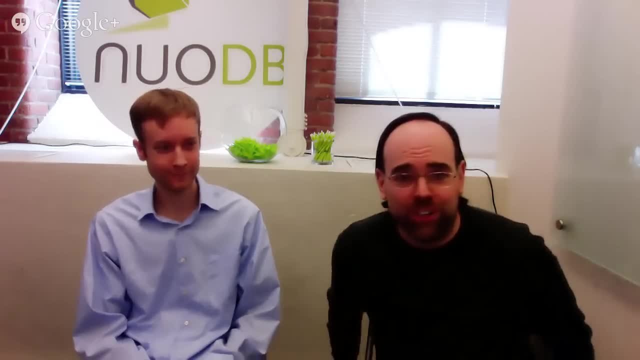 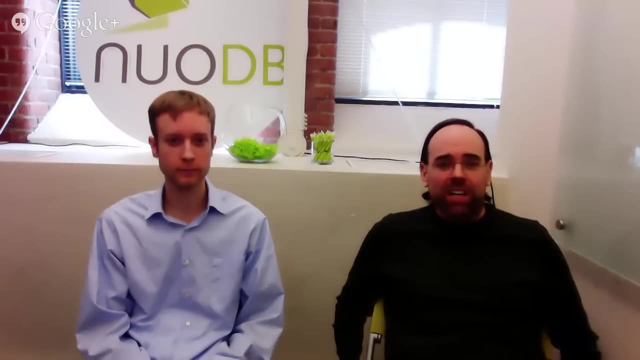 It's a really, really cool company. They are French, you know They do very cool technology And we're really excited to be working with them. We've been having a really great time working on this project. If you're curious to learn a little bit more, kind of about not just what we do, but kind of who some of our customers are and why they love us, go check out the website. 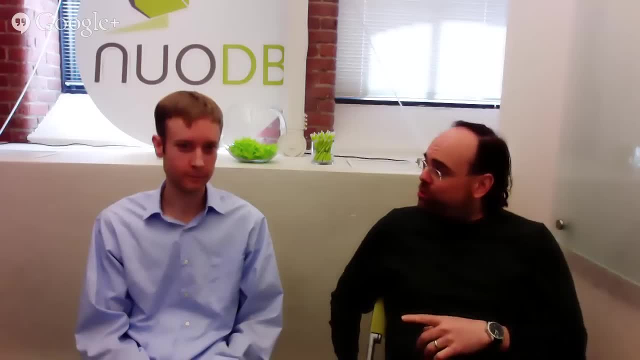 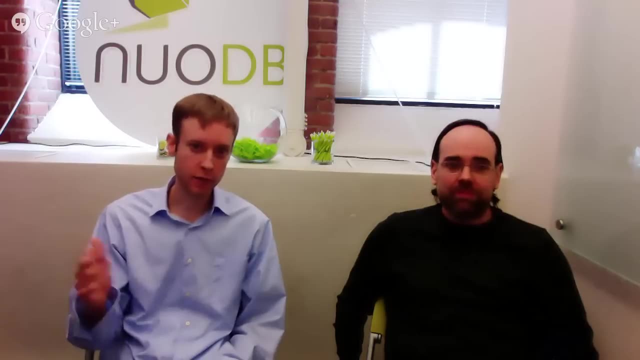 All right, Enough of that, Ross. you want to introduce yourself. You want to tell the folks at home who you are, where you came from, what you're doing here? Sure, I'd be happy to. So my name is Ross Shaw. 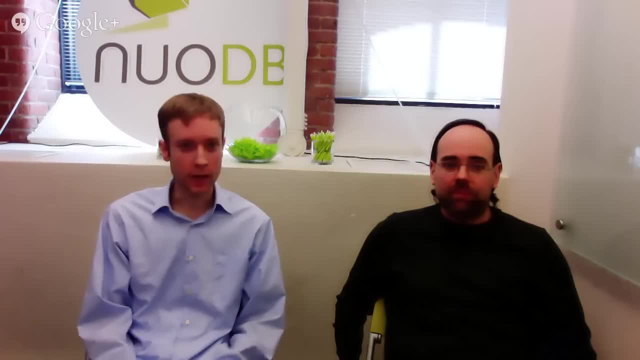 I'm a core engineer here I came from. I guess Brandeis University is the last place that I was before coming here In fabulous Waltham- In fabulous Waltham, That's right, Not too far from NuoDB headquarters. 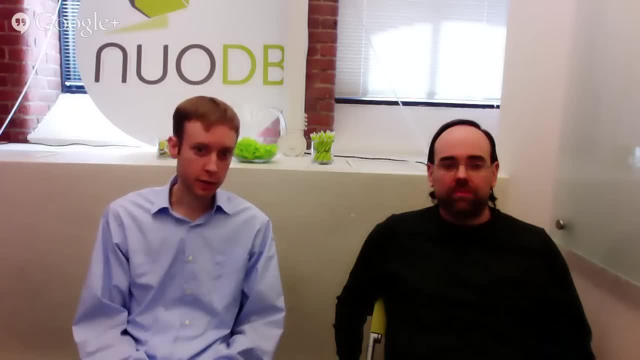 I was last working on my dissertation, which was a system to add a database, a modular layer for database snapshots and time travel. So basically that was all about figuring out Sort of a systematic way to provide this time travel capability within an existing database system. 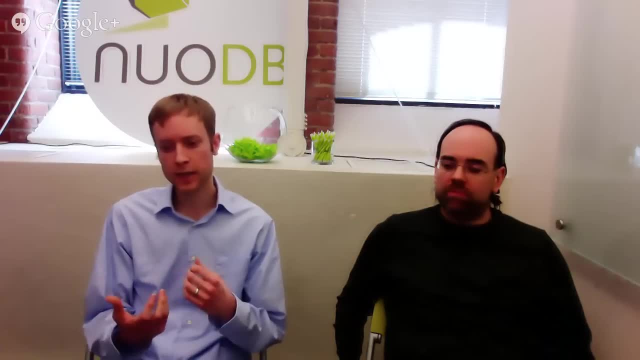 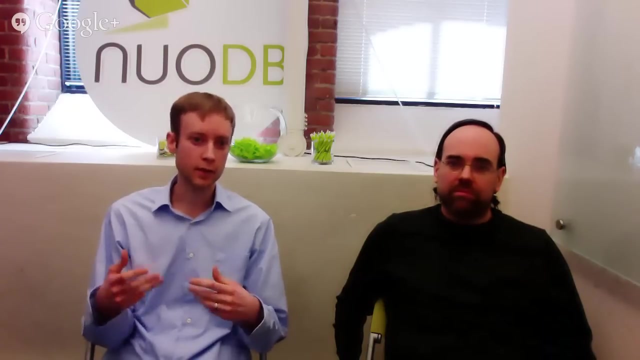 So really the magic there is: how do you take a system and say what is sort of the best way to add high performance snapshots that are transactionally consistent and can be saved sort of with any frequency that you want. However often you are committing transactions, that's the frequency with which you can save transactionally consistent snapshots. 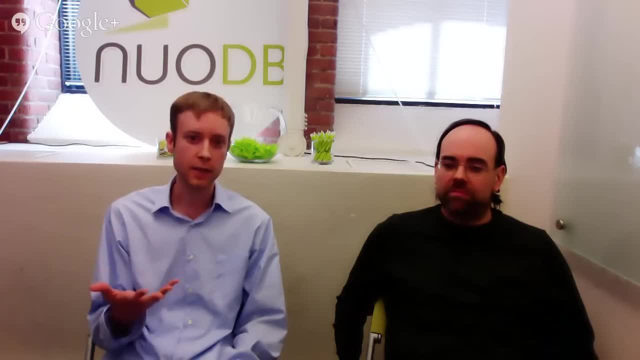 And then in situ, that is, within the same database, go in and perform queries as of any snapshot that you've declared. So that was really what my thesis was about, And it got me interested not only in database systems in general but in how you go into existing databases and, in a modular way, provide that data. 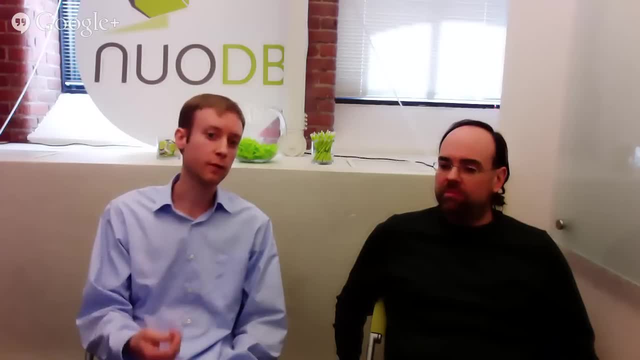 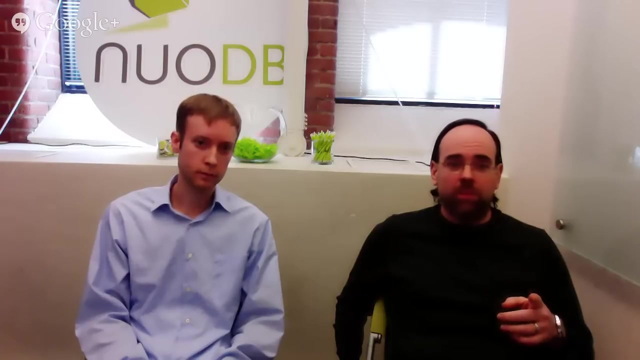 Right In a modular way, provide new high performance capabilities that sort of. provide new features and new capabilities that enhance both the performance and the correctness of the system. Nice, So what I said, Smart database guy. So very cool. And for those of you kind of playing along at home who don't have kind of the technical background that Ross did, 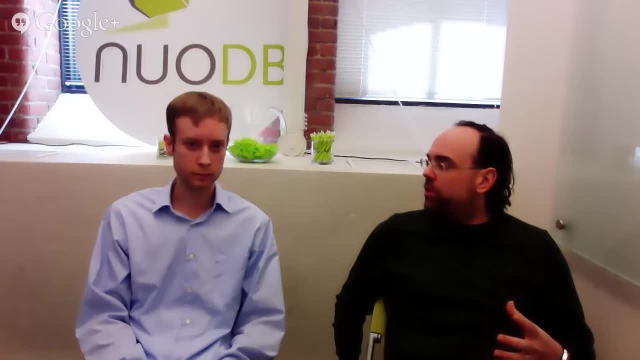 Ross, I think kind of what you were describing was this: gives you a great deal of flexibility, Right In terms of pragmatic features like the ability to do restore transactionally consistent fashion, the ability to reason about the state of the database at different points in time, kind of solve those kinds of problems. 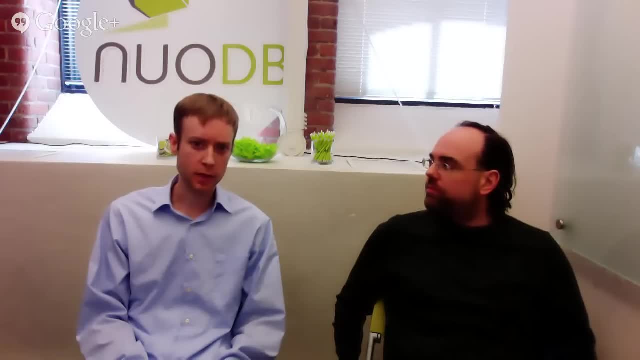 That's right And in fact one of the technologies that I used, that I in fact relied on quite heavily in my thesis, was MVCC, an optimistic concurrency control protocol that is widely used in databases today. Most practical databases support it. Lots of practitioners use it. Rely on it for efficient transaction performance. Really, what it gives you is the ability to go and perform reads while writes are, while updates are executing, And so that experience that I got relying on that for high performance snapshots also translated well to coming to NuoDB, because NuoDB, of course, is an MVCC provider. 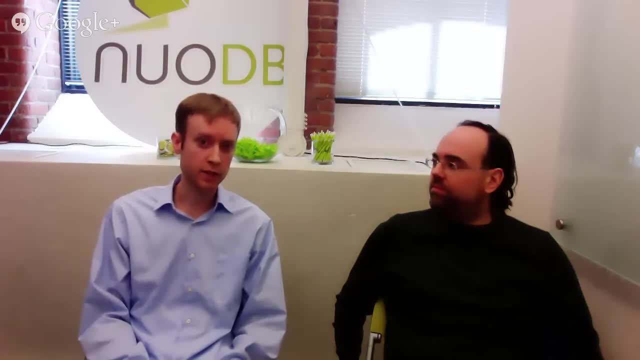 Right, We really rely on it. It's part of the NuoDB core full, All right, Thank you, Thank you, Thanks Ross, Thank you, Thank you, Thank you, Thanks Ross, Thank you, Thank you. 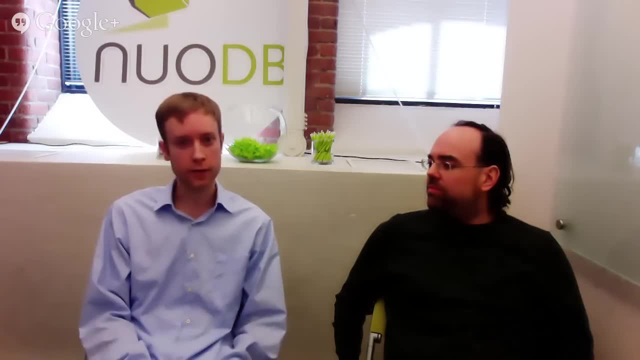 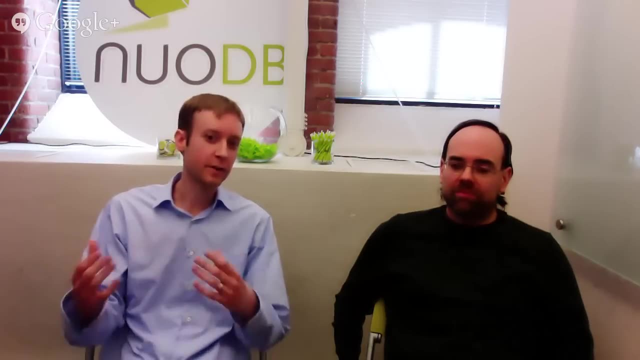 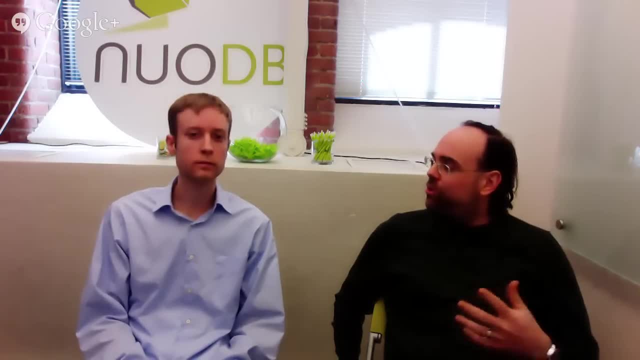 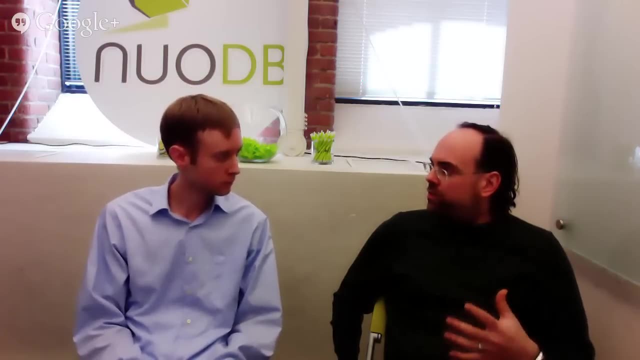 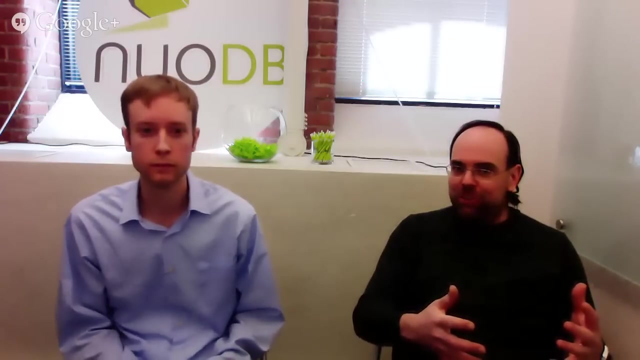 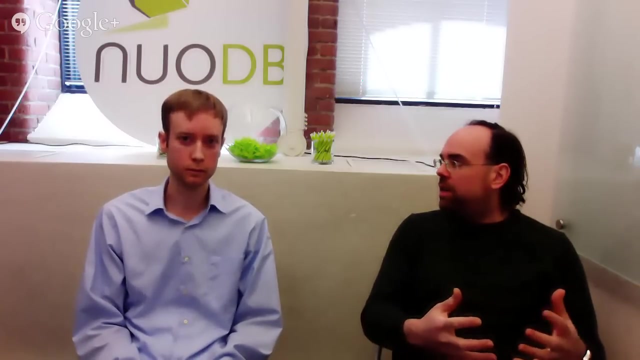 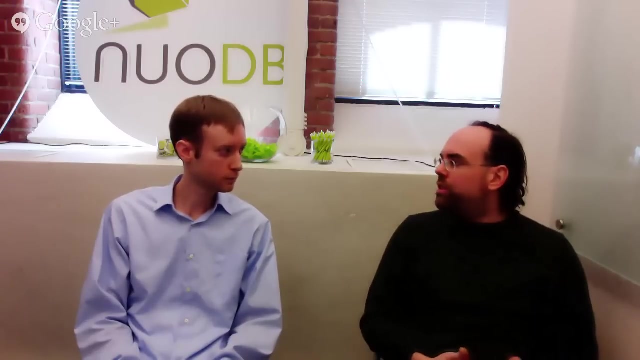 Thank you. And then we have a bunch of questions to what a distributed system looks like and kind of what the differences are. Yeah, So kind of what's your early experience? You've been here six months, seven months, something like that. 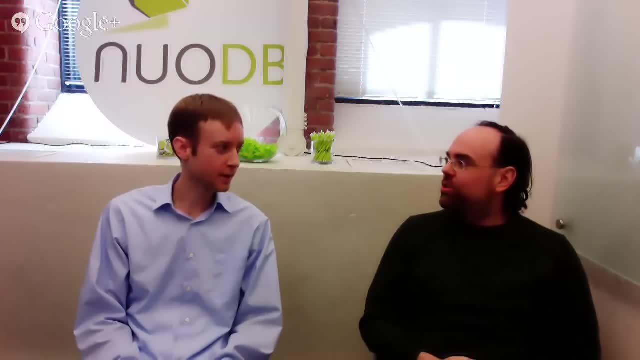 Yeah, over six months, it's yeah, something like that, yeah, And so what's your kind of initial take? What are some of the things you see that really make it? you know that are kind of distributed, interesting. 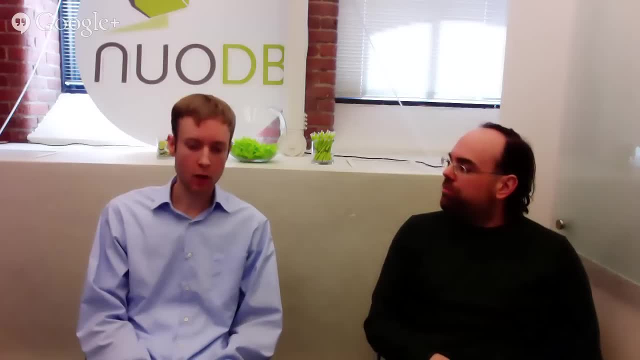 any challenges that you have in a distributed system like MoodBP. Well, it's certainly been a really interesting challenge, sort of coming here and applying what I learned. you know sort of what I focused on in my thesis- and single-instance database problems and applying them to a distributed database. 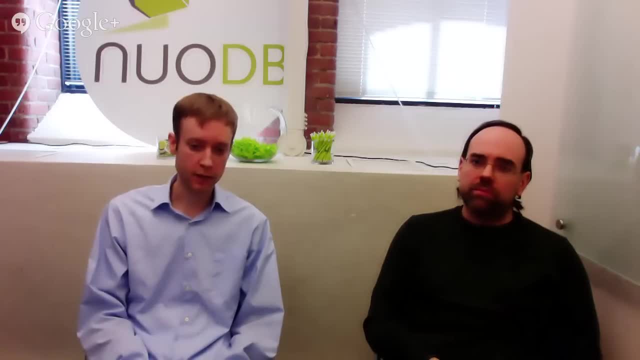 And I would say that you know my initial experience is I've definitely been having to ramp up quickly applying what distributed systems knowledge I had, what I learned in school or just from previous experience, and applying them in a database context. So some of my first projects involved, you know, for example, 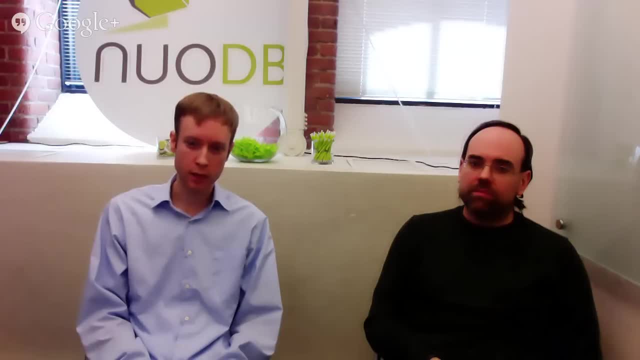 taking a protocol which may be familiar to anyone from the database community who's maybe worked in just single-node databases like something like Quies. One of my first projects here was sort of working on the Quies protocol that we have in a new ODD. 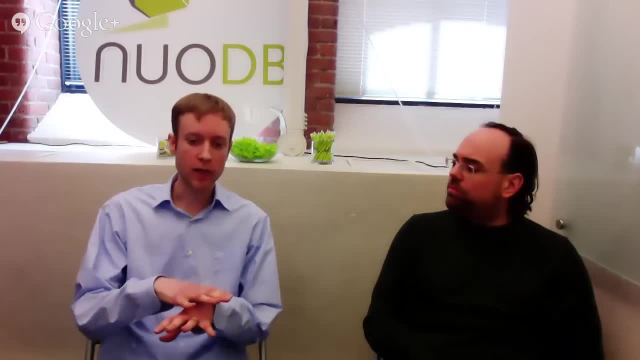 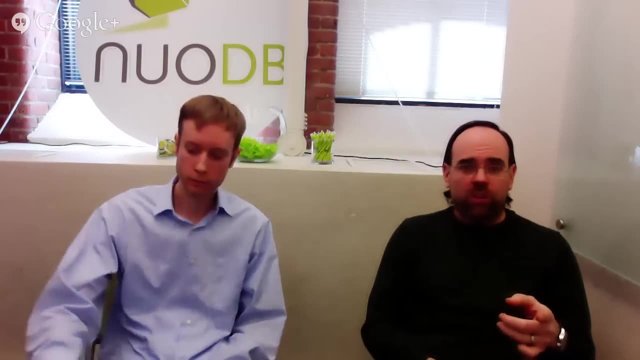 and working on a protocol to apply that to the, to everything, Every node in the database, right, Right And folks at home. probably most of you know what Ross is talking about. But Quies is basically saying to a database: keep running, like, keep the process running. 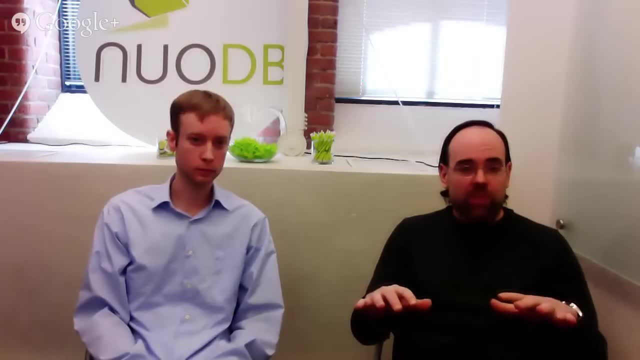 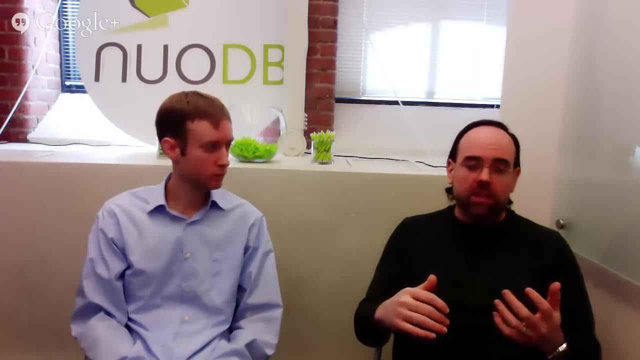 keep kind of all your state going but get into a quiet, stable state so there are no more transactions running, It's not doing any work on behalf of the client, So you get into a stable state. that's useful to do diagnostics, to do reasoning about the state of the system. 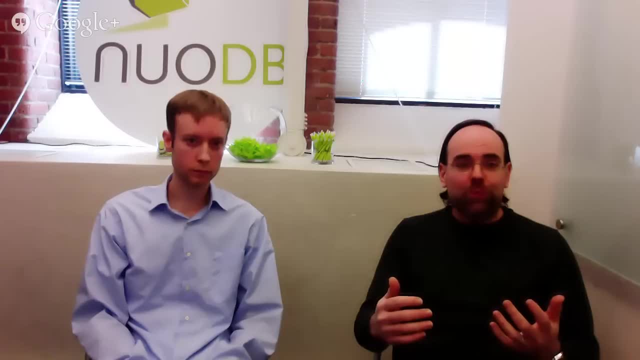 maybe to do a backup. So it's kind of a common feature you'd want to do in a database. It's a little bit easier to think about, you know, when you have just one process running as opposed to maybe dozens or hundreds of processes. 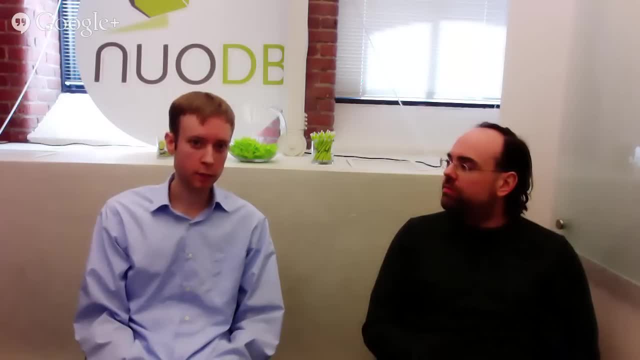 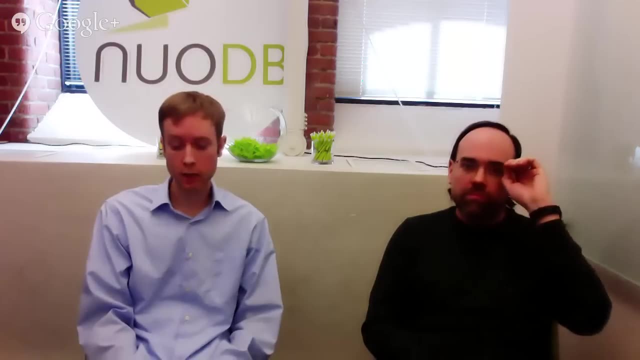 Right And, in particular, it's also generally important that a Quies database not be doing any IO. If you want to go back up- for example, you mentioned doing backup during Quies- It's probably important that your database not do any IO. 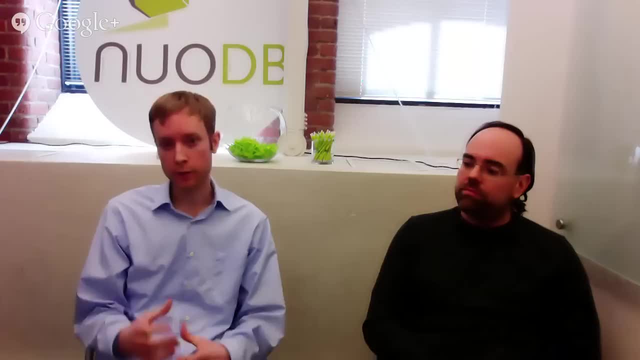 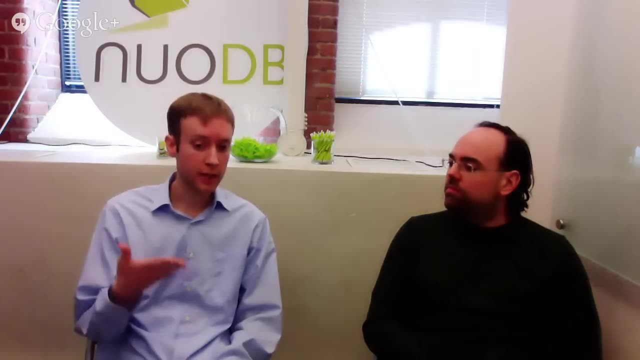 You may know that if you want to go and do a backup where you're, as you say, take a copy of the actual database files on disk. if the database is doing IO during that time you- your database may actually be. the copy that you create may be in an inconsistent state. 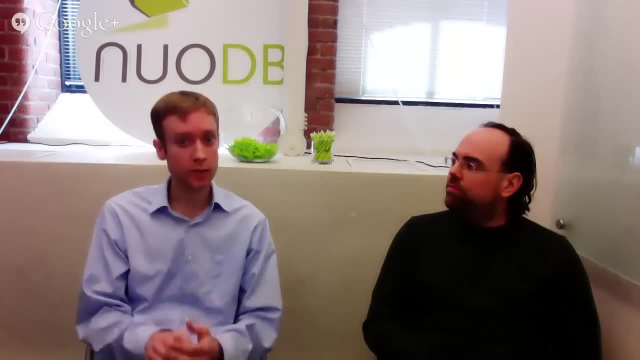 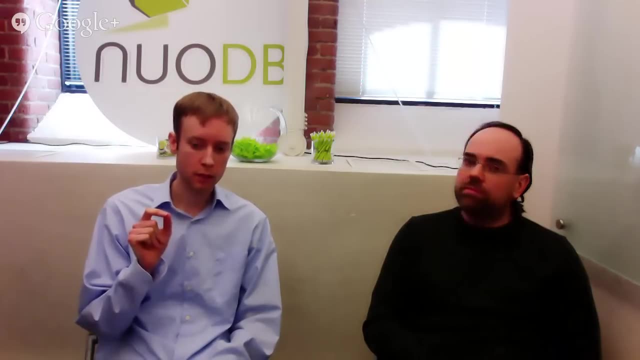 So you want the QES database to not be doing IO. So if you stop transactions from happening during that time, you will be preventing IO. but also you have to actually stop the GC process from happening, the garbage collection, because while garbage collection is happening in any database, not just in your DB- 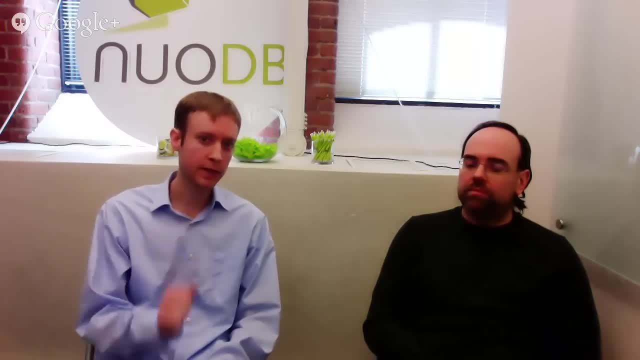 it may evict objects from memory and write them to disk if they're dirty. So the QES protocol not only has to stop transactions from coming in and issuing new updates, but also it has to flush the garbage collector and sort of quiet the entire system. 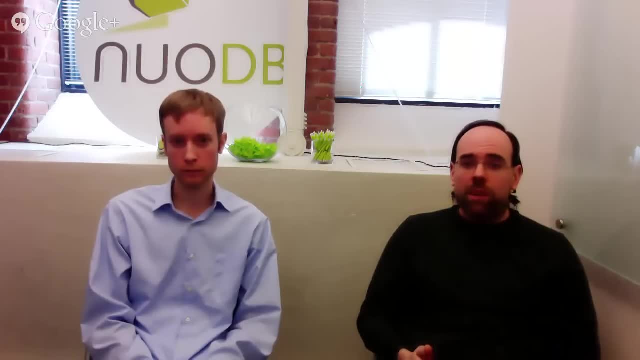 And of course in NodeDB we make it easy to do a backup without having to QES the entire database, because you can take a single kind of storage point offline. you can leave the rest of the database running Exactly. So for us. 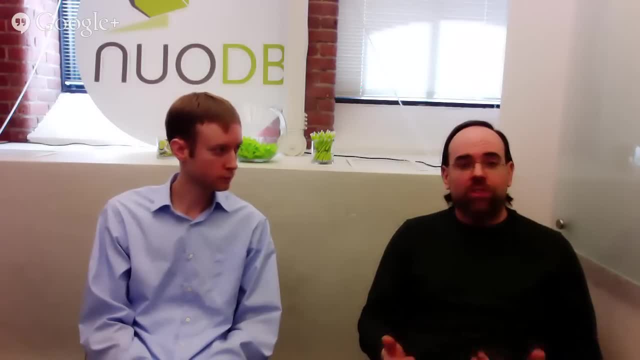 QES isn't as important for the backup cases but, as Ross mentioned, there are a number of other reasons. You might want to get into a steady state, be able to understand something about the garbage collector, understand something about how the system is behaving as a whole, to be able to do maintenance. 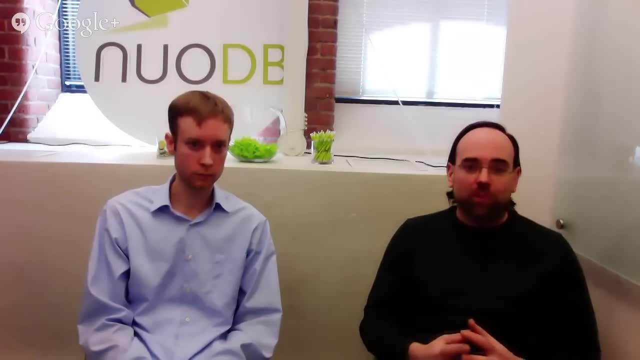 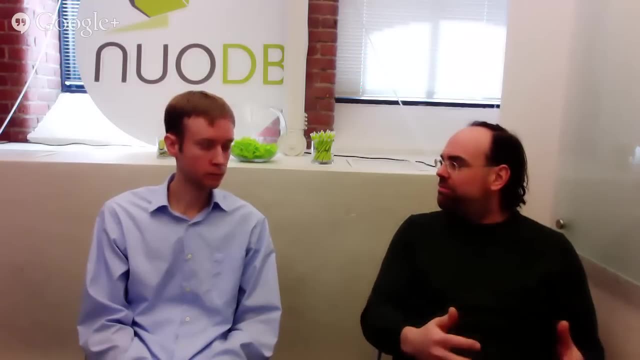 There are any number of reasons why you might want to address that kind of problem Exactly. So that's kind of interesting. So you've got to kind of think about how a traditional database problem gets multiplied or affected when you work across a distributed system. 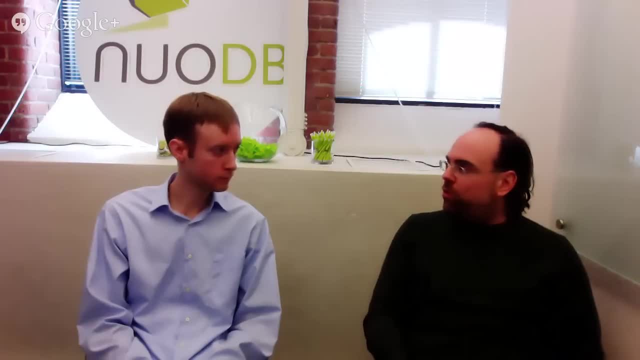 Correct. Now, in addition to kind of those traditional database problems, you've been spending the last few months kind of really digging into kind of more of a traditional distributed systems problem, Right? So what I've been working on lately is a problem that sort of. internally we refer to it as the node list. 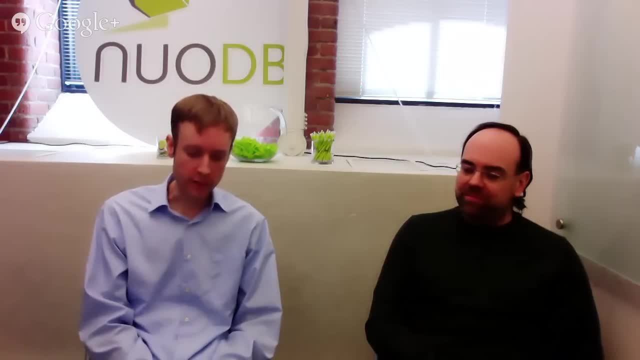 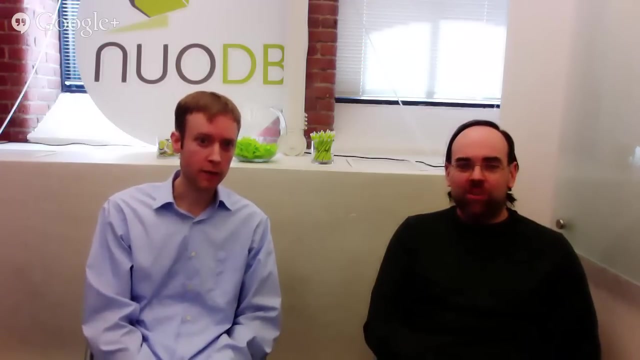 So I'll be using those words. It's really a problem about both membership and leadership. So those of you who are familiar with distributed systems, as soon as you hear leadership- probably some you know alarm bells or some lights will go off in your head. 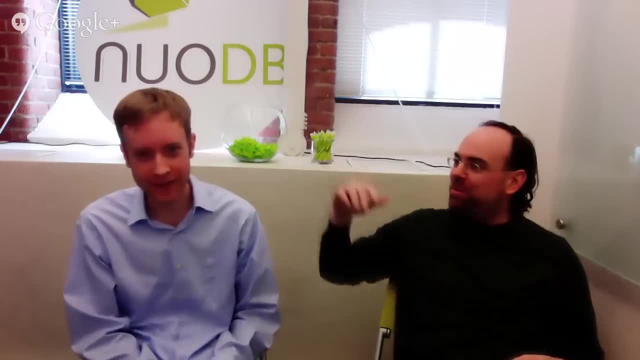 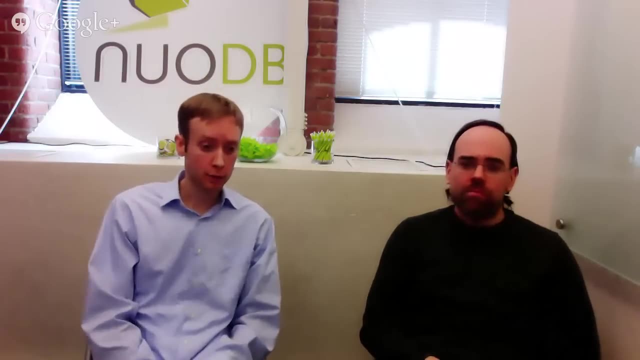 This is the time when we should have Google Hangouts, like put the like the thing over your head. Yeah So, and that may- even just mentioning that word may generate some questions, So I'll try to be careful in the language that I use in talking about it. 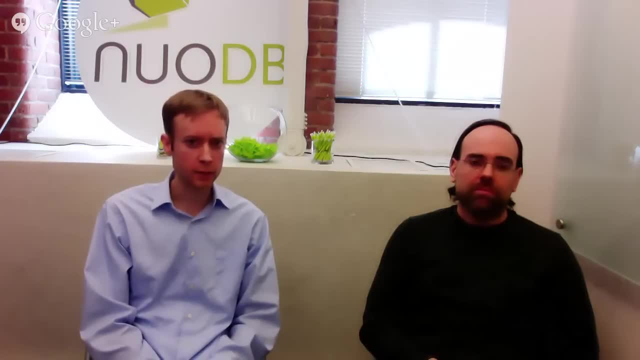 NuoDB uses a slightly different word to talk about this notion of leadership. We refer to it as chairmanship. The reason that we do that is we want to distinguish. We want to distinguish a little bit the way that we do leadership as compared to most other distributed systems. 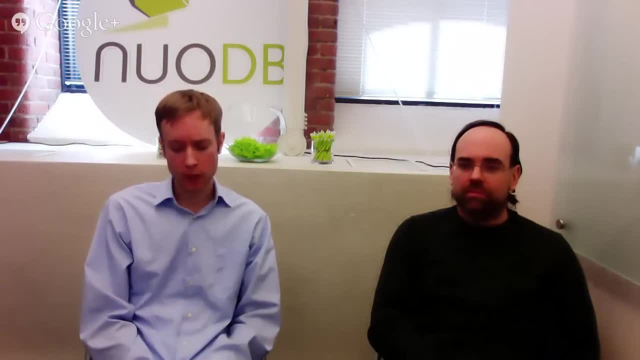 Let me define it in just a few little terms. In NuoDB we have a it's sort of like a big distributed cache. in a way, We have many different nodes in the system: TEs and SMs. For those of you who don't know the SMs, they're the storage managers. 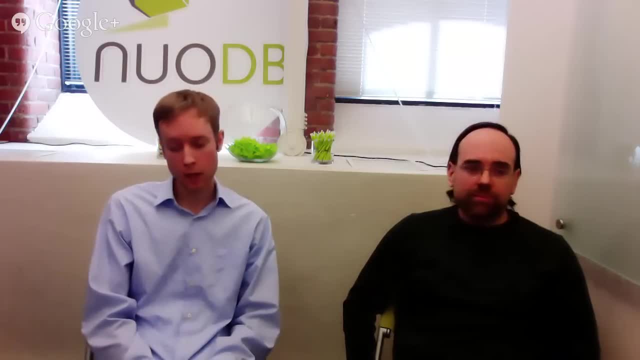 these nodes that actually have storage. They're attached to them. And then the TEs. these are the they're called transaction engines. These are the nodes that help us essentially scale out. They perform queries right. You submit a query to the NuoDB database and the TE will perform it for you. 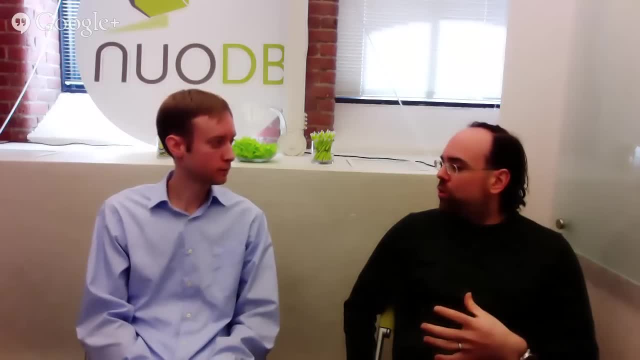 And these are in-memory processes. So part of why you're working on this problem is because these are essentially caches. These are coordinated caches, Correct. Each of the nodes has its own local cache, of course, in memory, in RAM, But the 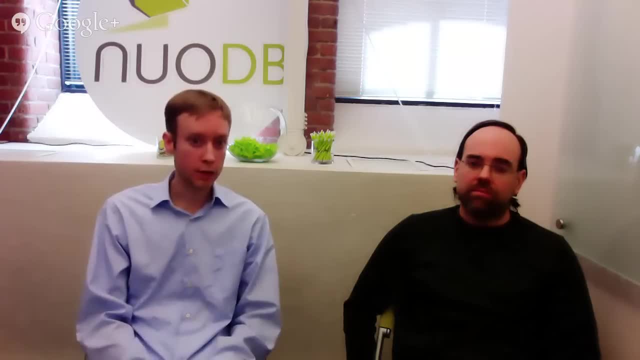 NuoDB database as a whole is a big giant cache. All of the caches are have to coordinate. It's a distributed cache. So each atom in an object that NuoDB database tracks it lives, it has a home in storage. 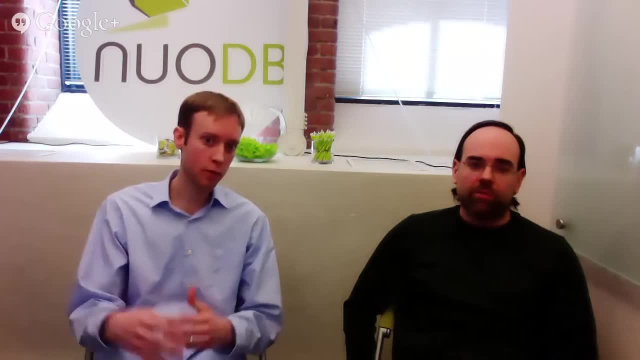 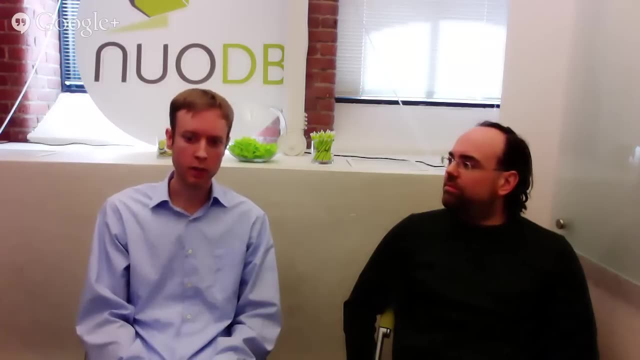 and in SM, but it's also cached at zero or more nodes in the database. It may be cached nowhere, but usually it's cached somewhere. If you're querying it or updating it, it's going to be cached In a TE and in in in uh SMs. 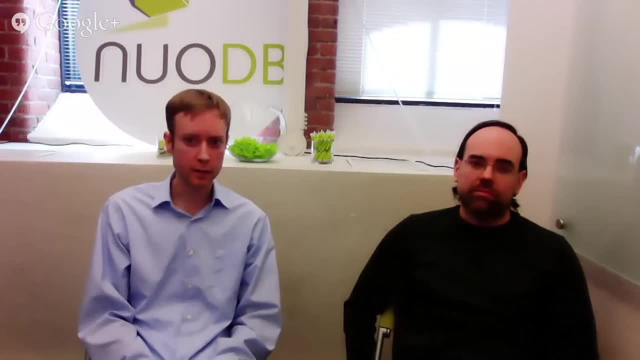 And the locations where it's cached has to be uh tracked in. a. a membership set Uh, and there's multiple reasons for this. Uh. one reason is because we need to cut down on the number of uh replication messages. 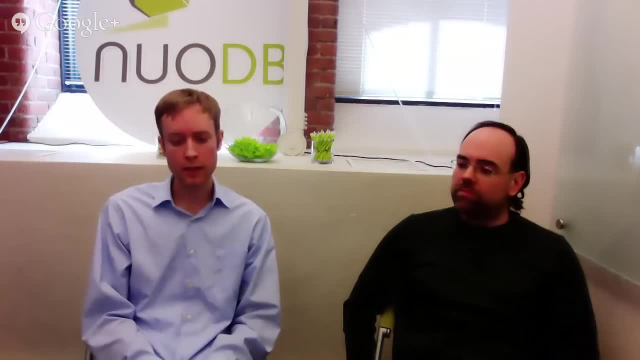 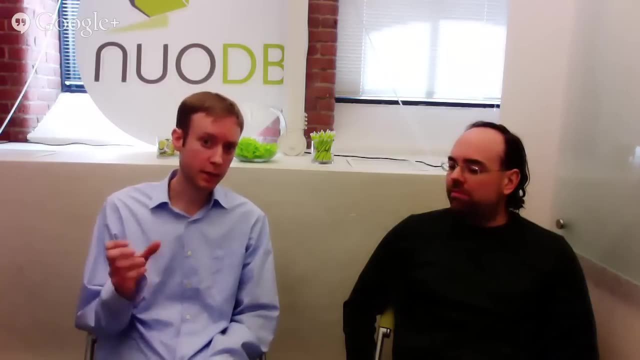 that we send, So distributed systems. they need to. when an object is updated, they need to tell the other uh nodes in the database that this update has happened. Basically, you know if you, if you do an update to an object. 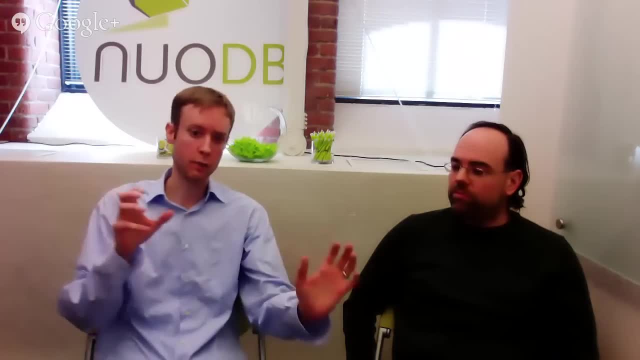 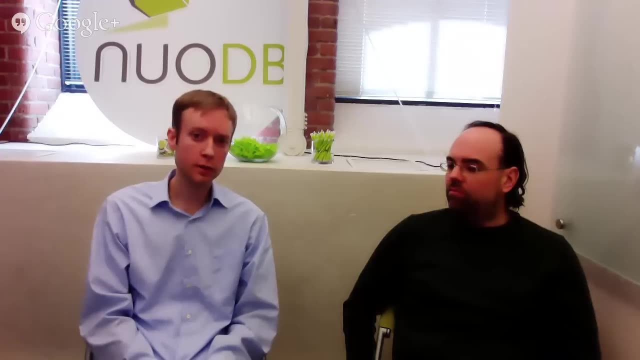 If you do an an atom, you need to tell the other nodes where this atom is cached. if this update has happened- Uh, we do this with group replication message. If we didn't know which nodes were uh caching the atom, it would be well, it would be difficult. 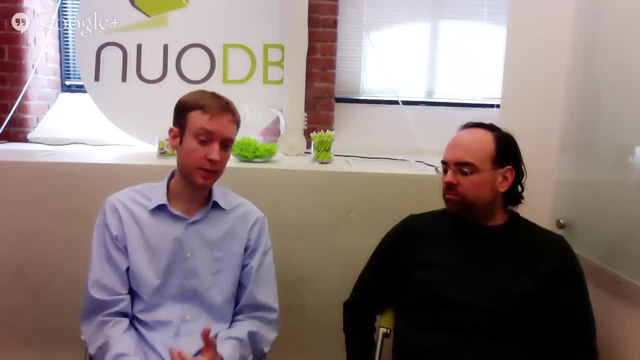 to to tell them, but certainly you can imagine that you would have to to tell every other node in the system about it. So you would have a essentially an you know you have to tell, send a replication message to every node. 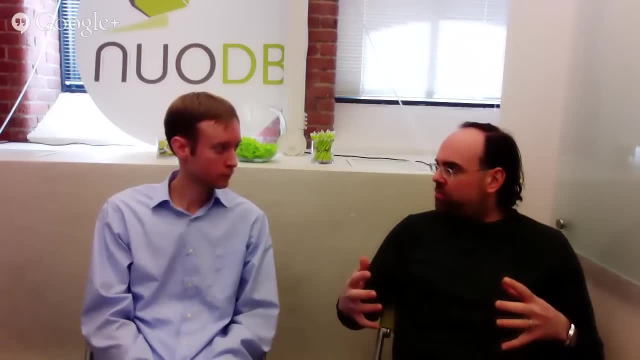 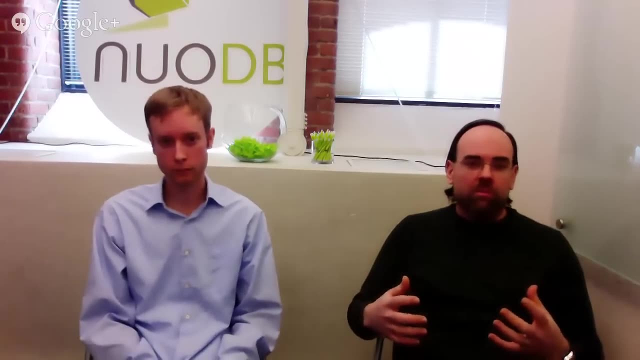 So this would be very expensive. So so you're describing, kind of: we've taken the database, We've broken it up into what we call atoms, which are chunks of data that represent a particular role, Uh, a block of data representing an index, or the data itself, or metadata, schema data. 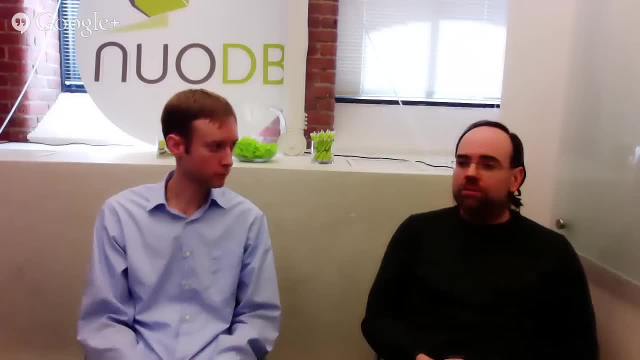 something like that. Right, So we have atoms and then we have these transaction processes that are in memory, that are caching at the granularity of an atom. Correct, Some transaction engines have one set of atoms. Some transaction engines may have a different set of atoms. 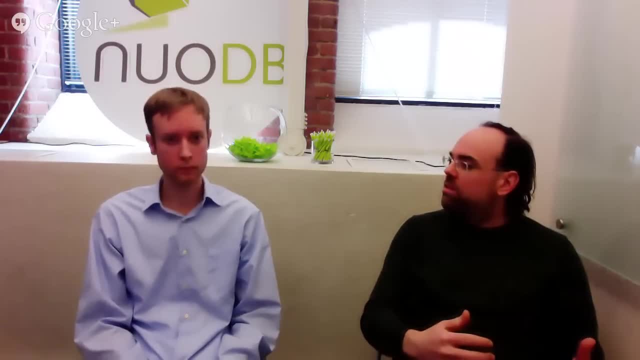 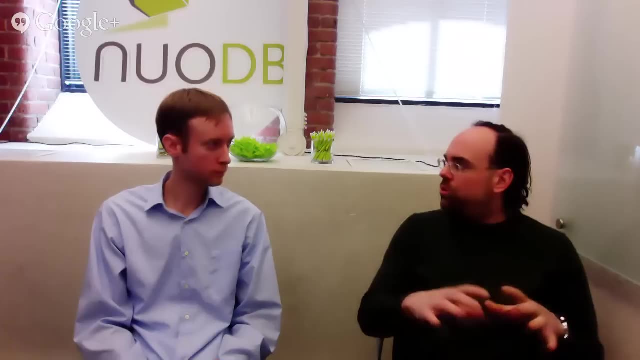 Some atoms may be replicated in memory in different places or may only exist in a single transaction engine. Correct, And so the the. the problem you're describing is, kind of loosely, that we have both the need to coordinate so that when we're making changes the caches are being maintained correctly. 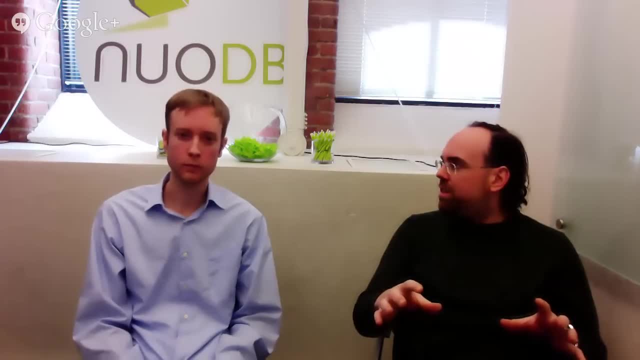 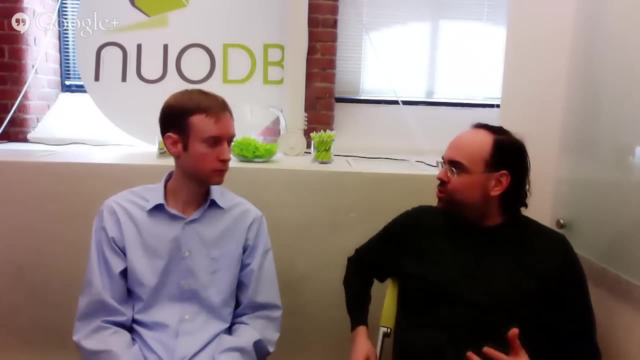 but also we need to make sure that consistency is maintained Right, So that if you're doing an update, that update is is is being handled based on the rules of kind of what an asset transaction should do Exactly. So there's sort of two points I can jump off from. uh, from that. 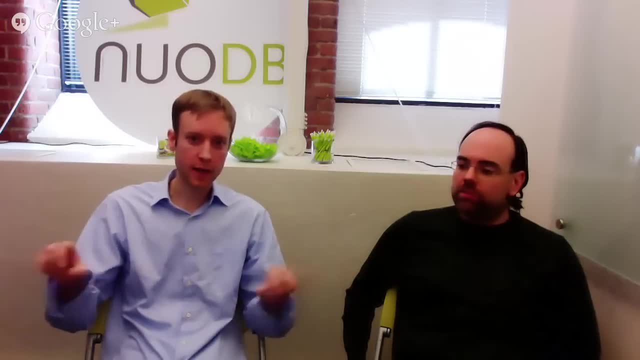 So you know, first of all, you mentioned that, you know, sitting on top of this atom cache layer are are many other layers that where we actually deal with, um, you know, SQL-level consistency and executing transactions. Um, you know, I think this layering design is very important. 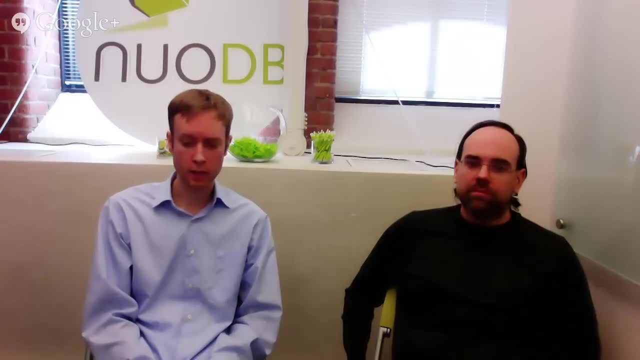 It's also, you know, sort of a a core part of how I look at systems, um, and, and I think it's, it's very important to system design to be able to break up, um, you know this. 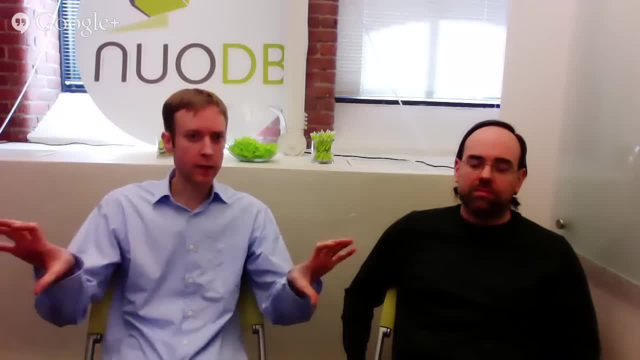 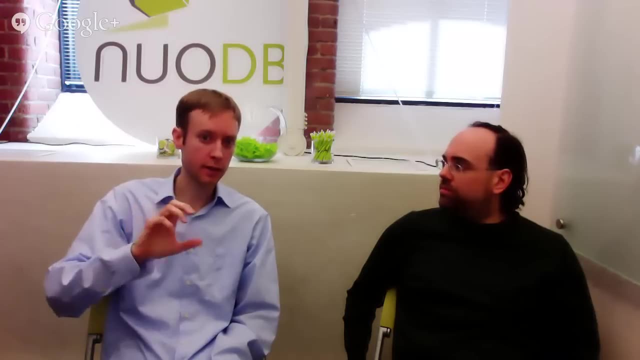 sort of uh storage-type layer, which is what the atom layer is, from the layers that deal with things like SQL, Because this there's actually transactions that are executed and I I think this is a very smart way to, to, to design. 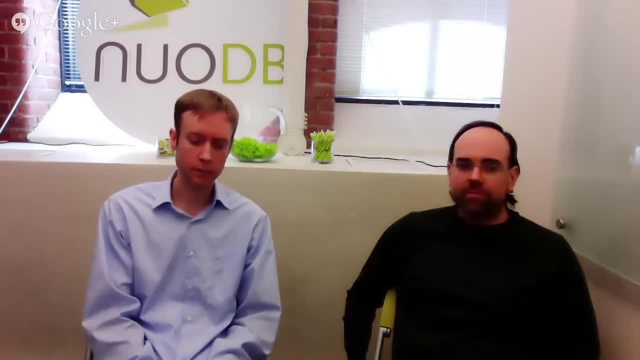 So that that definitely appeals to me on a system design level. Um, and so Seth mentioned: um, you know this coordination: if you're executing transactions, you're dealing with indexes. um, how do you coordinate those uh processes between atoms? 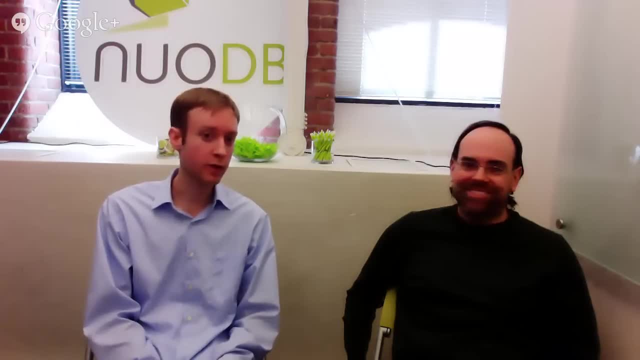 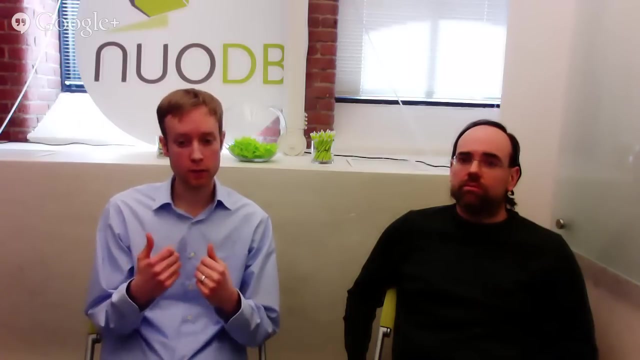 especially because usually- I guess always- they deal with more than one atom right. The way that this really happens is that when there's transactions that have to coordinate between atoms, and when they are, in particular when they're non-local, they have to go to a leader to coordinate those non-local actions. 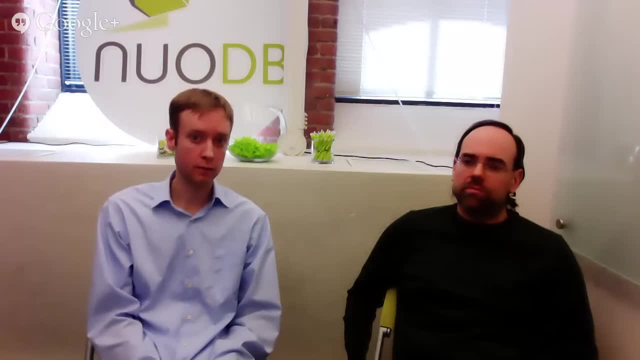 And they do this because there may be conflicts- right, You know that transactions may sometimes conflict. And they do this by coordinating through a leader, And we call this leader a chairman. Now, each atom has its own chairman. It's not like we have one leader for the entire database. There's not one single point of failure. Each atom itself has a chairman. 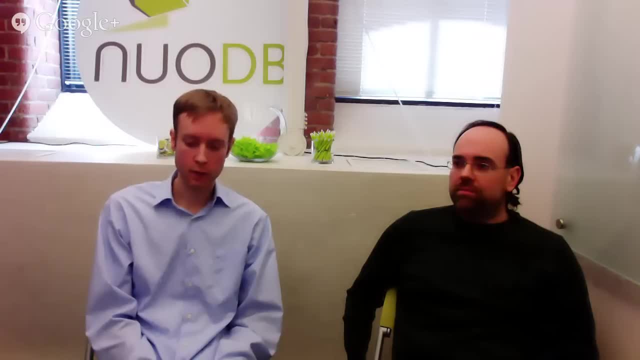 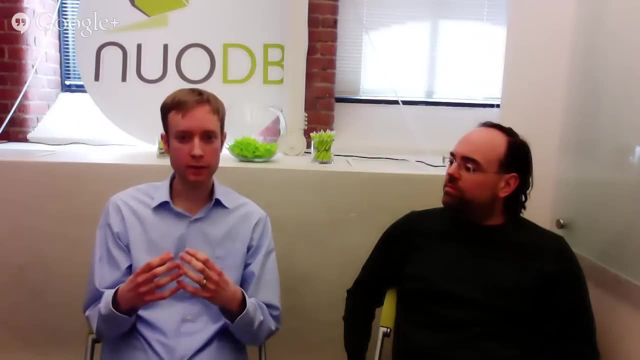 And the way that we do this is interesting. The membership set that we maintain for each atom is actually not just a set, It's a list. It's ordered And the chairman for each atom is the first element in that list. So when a node enters this list, it just gets appended to the end. 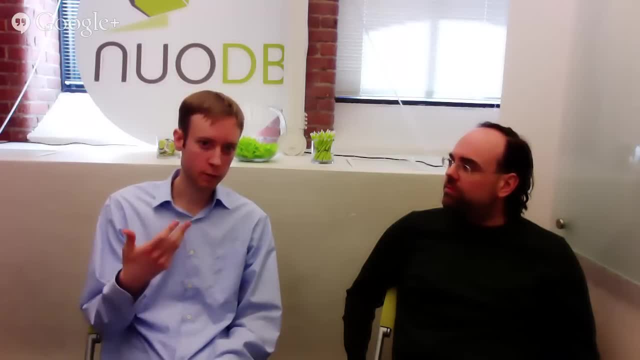 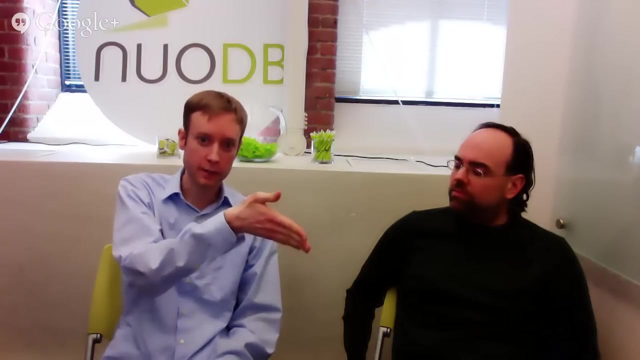 And when a node leaves, either because it fails or because there's cash pressure at that node and it evicts an atom, It's just removed from the list And the chairmanship simply is assigned by iterating. you know, it's just the first one in the list, whoever that node is. 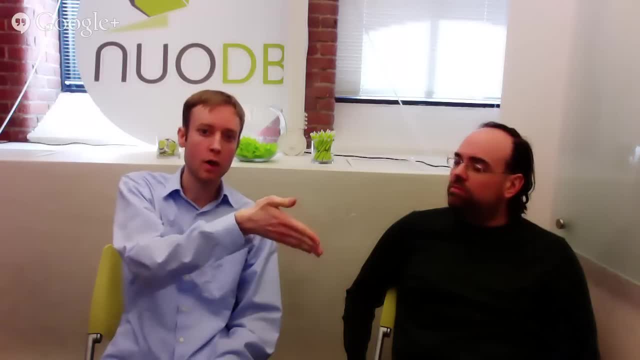 And if the first one leaves, maybe because it fails all nodes who are currently caching that atom? simply select the next element in the list. So our chairman selection, essentially leadership selection, is really very simple. So our chairman selection, essentially leadership selection, is really very simple. 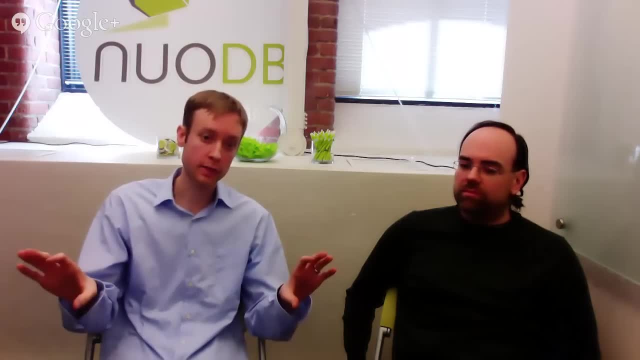 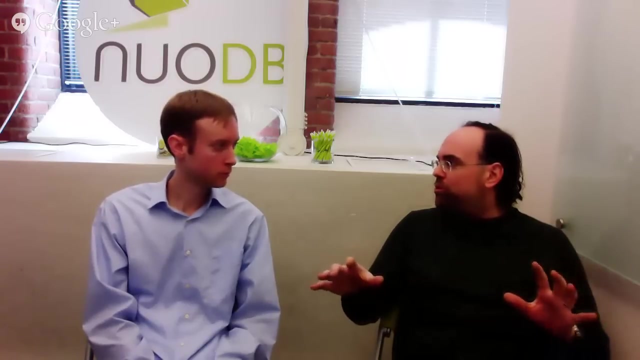 It just involves maintaining this ordered list And making sure that we always keep it up to date by removing nodes which have either failed or dropped the atom. So you're saying we've got these transaction engines distributed. They're all equal peers. there's no kind of central overload. 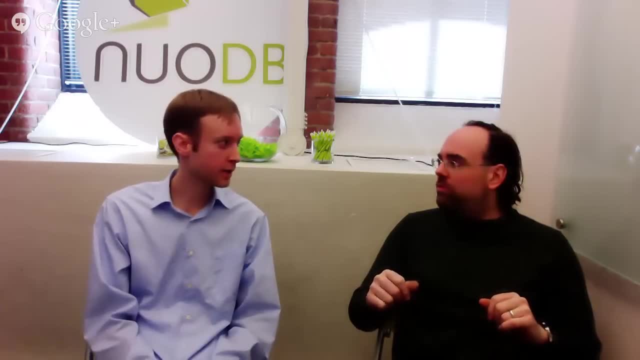 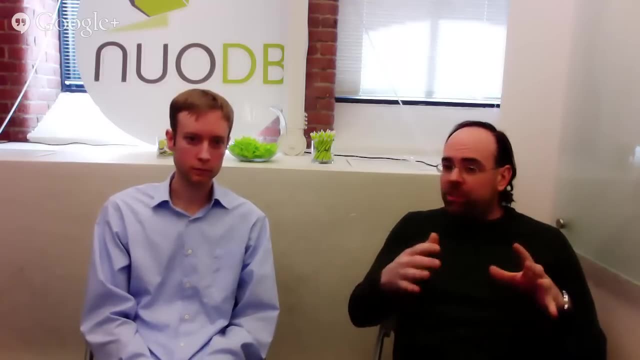 And it's important to note that storage managers as well. right, they have caches and they actually participate in the same way. That symmetry really simplifies the algorithm. We've got these peers in the system. Each of them has a subset of objects cached. 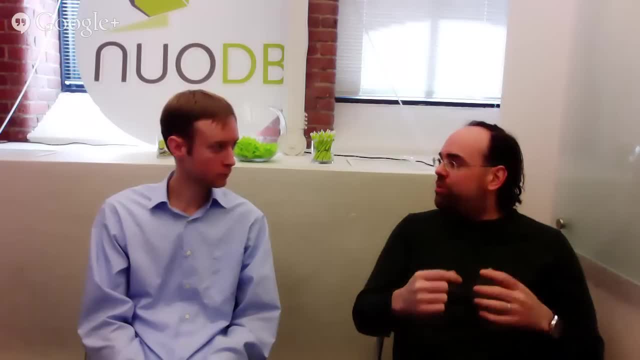 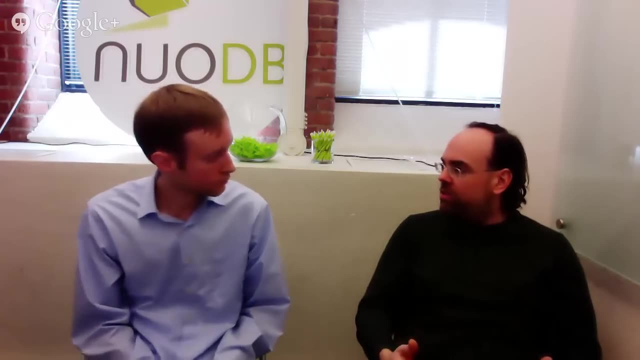 You're saying that for each of these objects essentially there's separate coordination going on to keep track of. if I'm a transaction engine, which of my peers also has this object essentially, And how do I know who's the authority for that given. 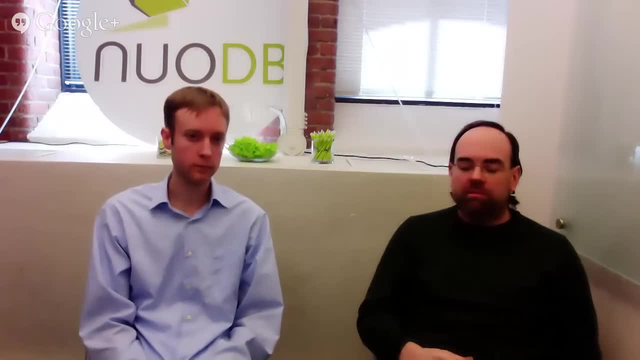 object at any point in time. Yes, correct, And so the idea here is that the reason we're not just running some global consensus algorithm or something is because really there's lots of atoms in the system. There are lots of independent roles being played. 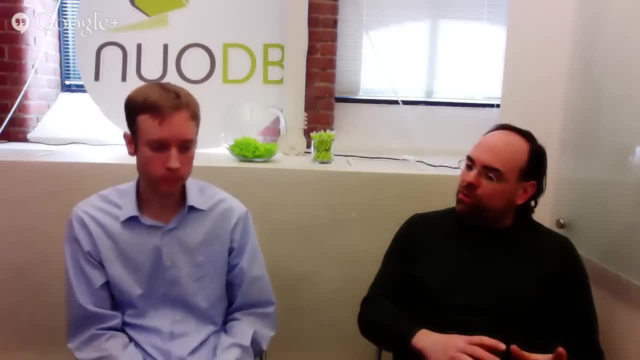 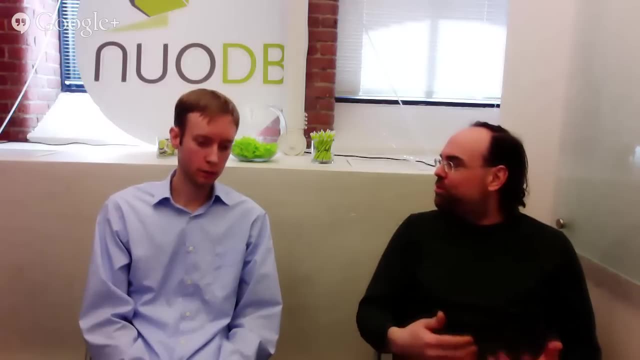 So there are lots of processes in the system which would be an authority for some things and not authority for others, And those roles are constantly being assumed and then drawn. So that's part of the nature of a distributed system, That's true. It definitely gives us a very efficient way. 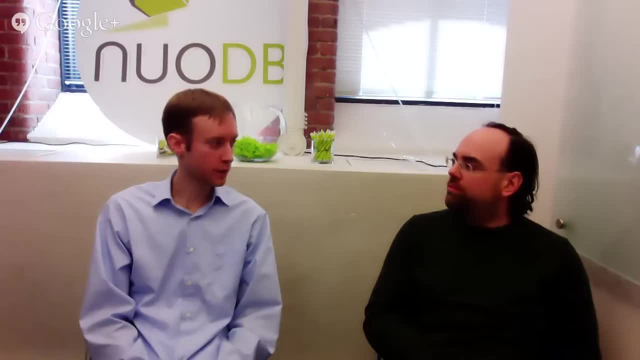 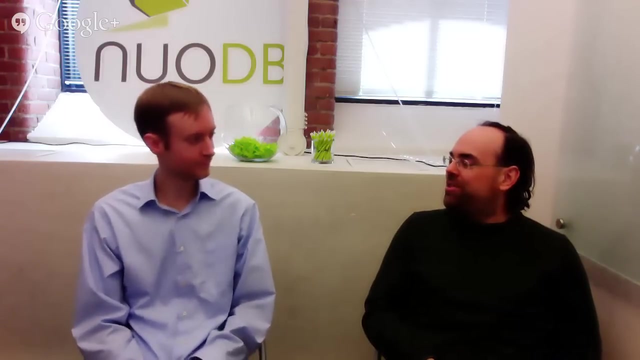 of choosing chairman on a per-atom basis- Cool. So we're doing distributed consensus coordination. That's really good. Is there kind of a next problem you're looking at with all of this? Is this something exciting, Or are you switching gears now and starting? 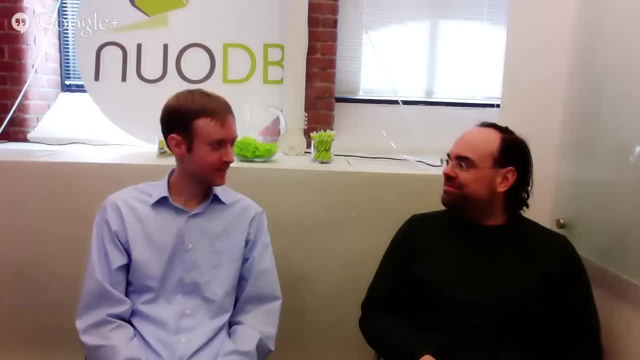 to look at new problems here at MootDV. Well, yes, Obviously there's always a next thing that we're looking at. So we have this big push right now behind always making this geo-better, bigger and better. So that's geo-distribution. that's running in lots. 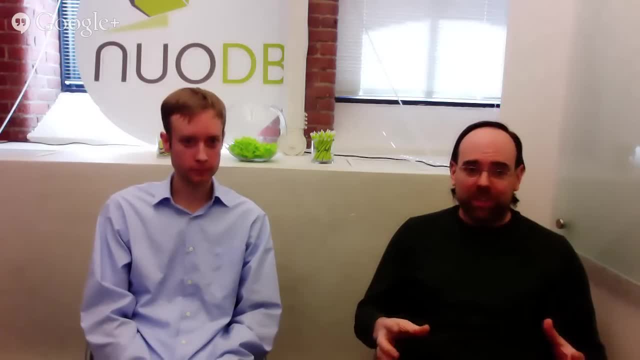 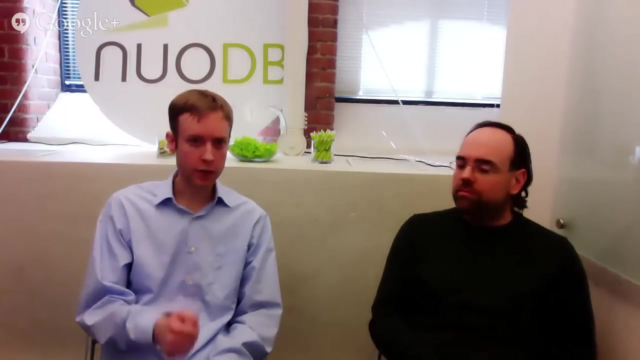 of different data centers running literally distributed around the world, a single database. So I have a project that I'm working on. It's jumping off of the node list project, But it involves making this idea of selecting a chairman more efficient when you have atoms. that 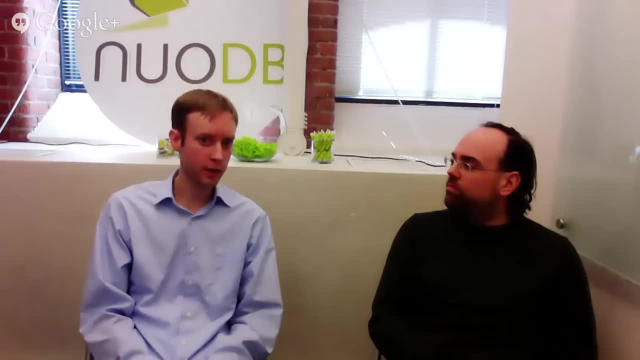 are distributed across geo-regions and not just data Just within one data center. So that's sort of the next project that I'm working on. Yeah, And for folks who are interested in learning more about this, we talk in our white paper kind of a little bit. 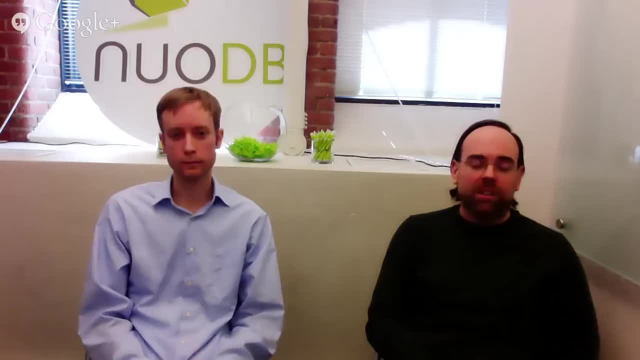 about how these problems work. We also have some information on our tech blog. One of the cool things that Ross is talking about there at the end is that this notion of chairmanship, this notion of who's the authority for any given object, follows from where atoms are in cache. 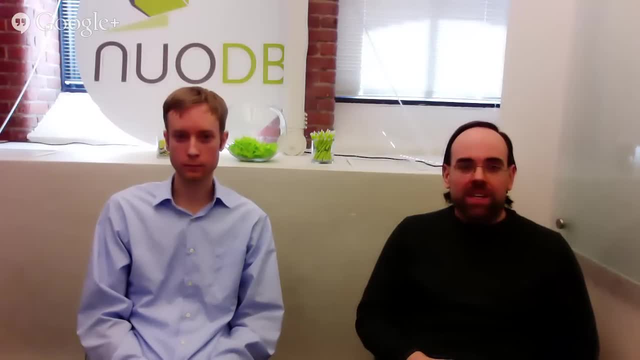 It's a very simple idea, And so because of that, if you know something about your access patterns in your application, you form natural affinity between your application and your caches And therefore you form natural affinity between these authorities and where data is being cached. 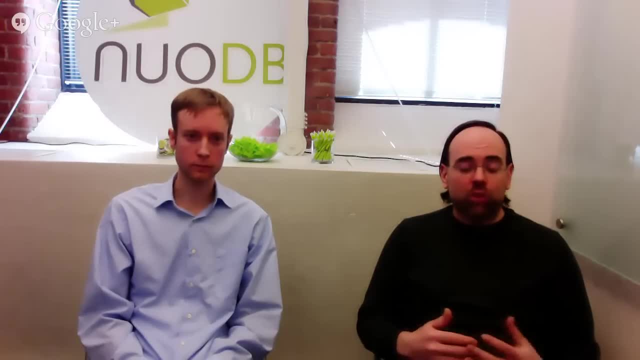 And obviously, when you start taking a system and distributing it across very wide distances, where there's lots of latency between sub-networks, making sure that you've got the right decisions about where things are being cached and where decisions can be made in terms of authority of objects is part of what makes it so that. 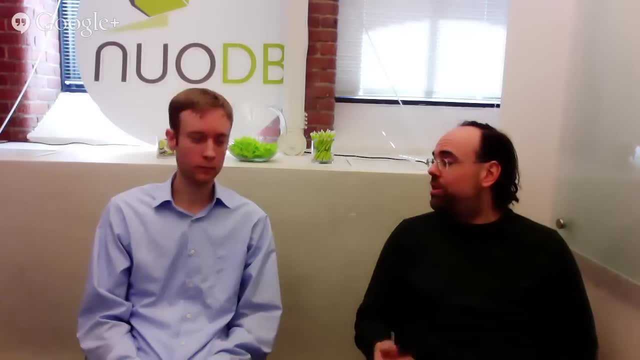 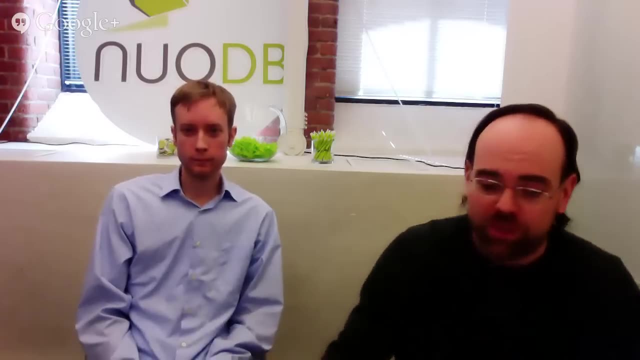 it's a good idea And I think that's one of the things that makes a system like NuoDB scale very efficiently and work really well. So that's awesome stuff. Yeah, Nice. We've got a couple questions coming in. I will try not to reach across you as I do this. 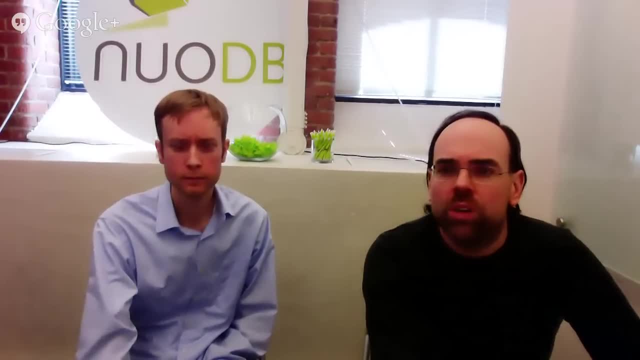 So Timothy asks. he says, realizing that distributed locking isn't the only way to protect data integrity, does your system use a multiversion system or locking system? What can you say about the memory overhead versus the latency costs of these, and why did you choose? 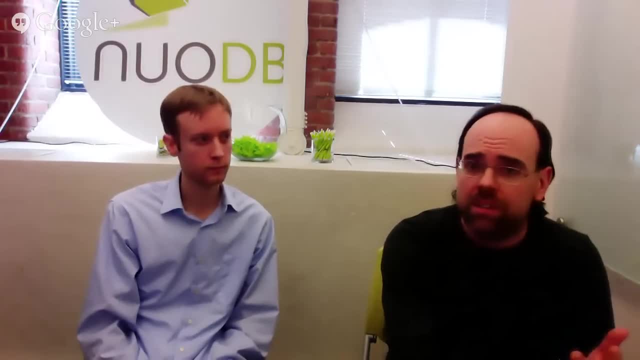 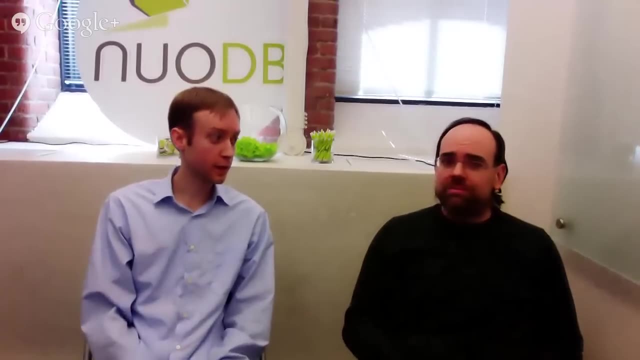 this course. All right. So you already talked about the fact that we're MVCC-based. That's a, So it's version control, But obviously there's still something around locking. Yeah, There's definitely locks. So the high-level idea is that we're 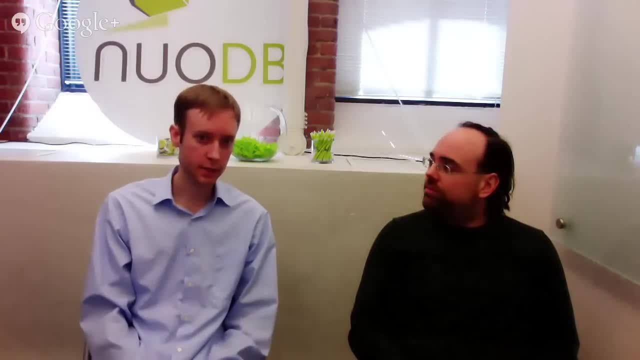 a multiversion concurrency control system, The transactions execute with MVCC. There is still low-level locking, sort of at the level of mutexes, if you think about systems programming. These are not locks. These are locks at the level of distributed system design. 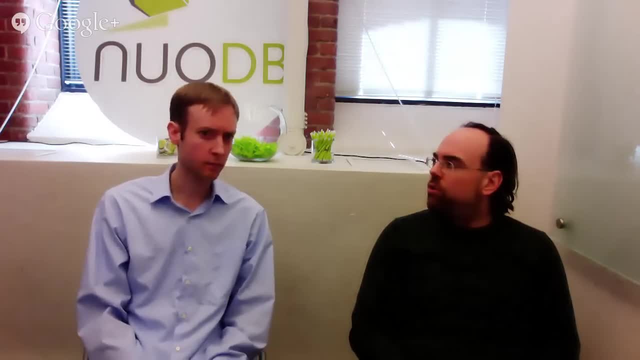 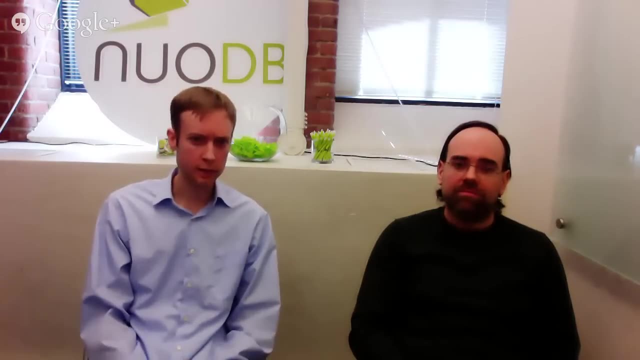 But obviously there's still locking. They're record-level locks, They're not distributed locks, Correct? Yeah? And in terms of memory overhead, I guess there is some memory overhead associated with having to associate mutexes with objects, But I would not consider that to be a particularly high memory. 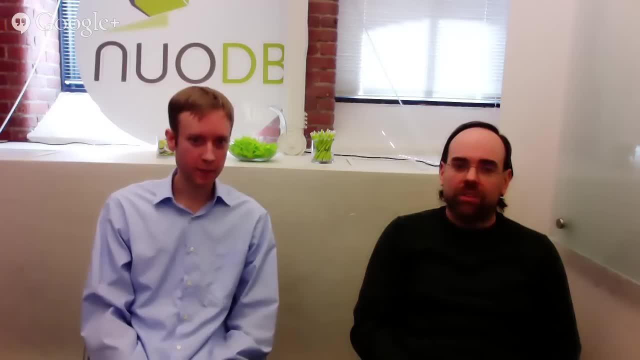 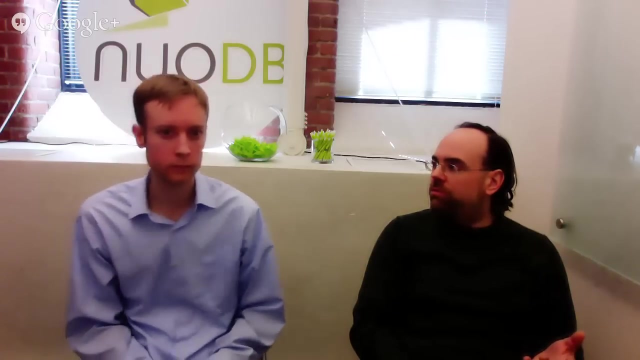 overhead. Some of my compatriots may disagree, But it's difficult to avoid. You do require some kind of mutual exclusion for coordinating threads and things like that. Right, And I think that's actually part of the point. you're right, This is both a saving in terms of memory overhead. 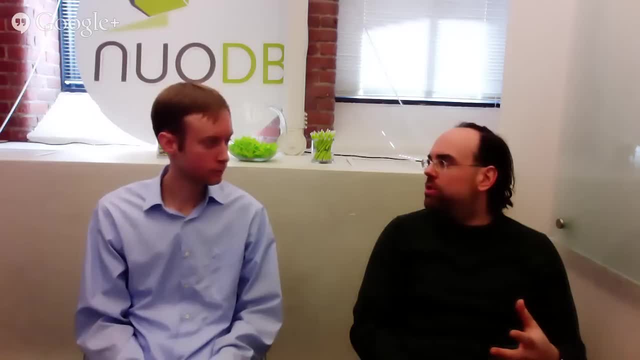 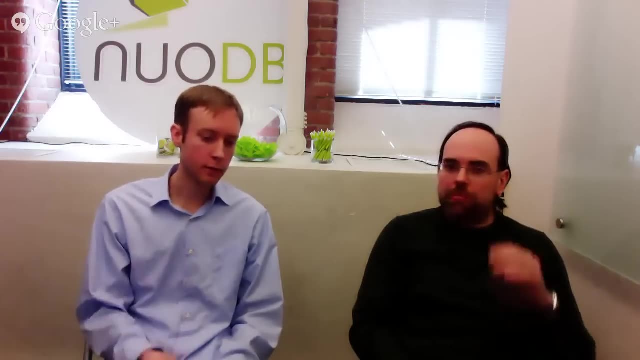 both in terms of the lock space but also the memory that would be required to do something like a distributed deadlock detection algorithm or some kind of distributed two-phase commit. That's true, And when you try to get rid of locks completely and go to a weight-free algorithm or something, 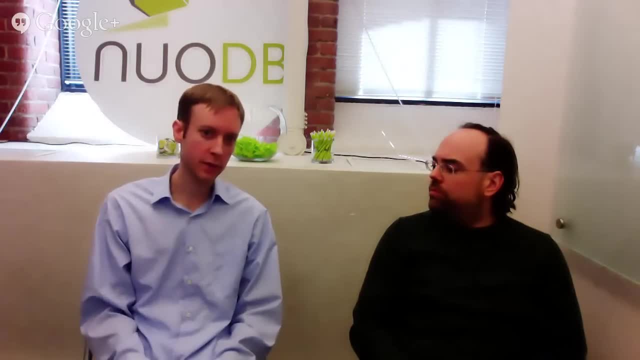 you end up paying a price in terms of memory overhead for those algorithms And you end up paying a price for those algorithms too. So there's always trade-offs in when you're trying to engineer these kinds of solutions. Right And Timothy, to your question of latency. 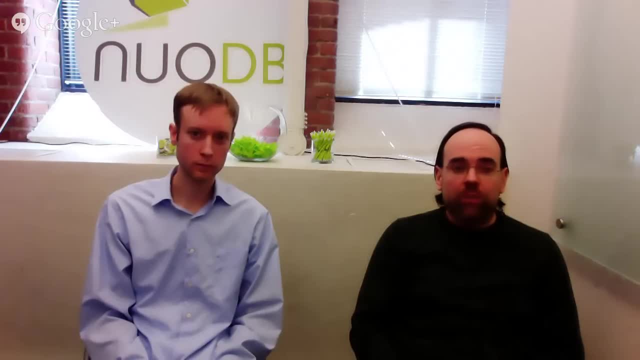 I think that's a lot of the point here is that what we build here assumes that you're running in a distributed fashion, that you're running across networks, maybe running across the public internet, certainly running between WAN speed locations, And so latency is really important to us. 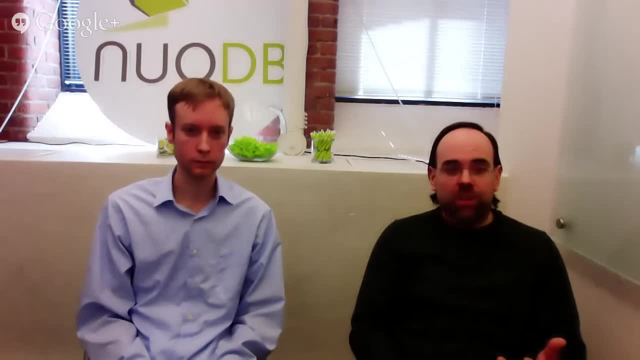 So a lot of our protocols- and Ross kind of touched on this earlier- are by their nature asynchronous and fairly optimistic, And that's part of what something like MVCC gives us is the ability to kind of start coordinating changes before we know they're canonical, to try to get ahead of network. 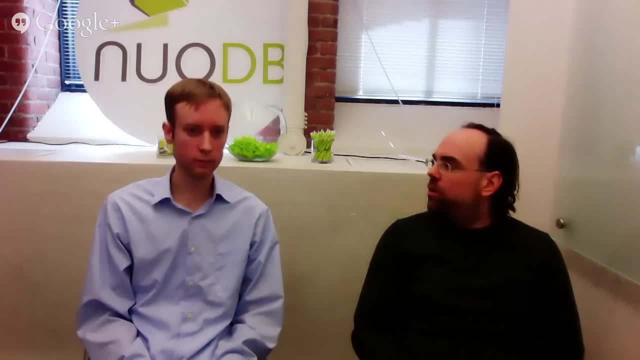 latency issues. That's also a lot of what these no-list changes are about is being able to very aggressively share information before you actually need it, so that you end up stalling less, you end up blocking less, you end up being much more tolerant. 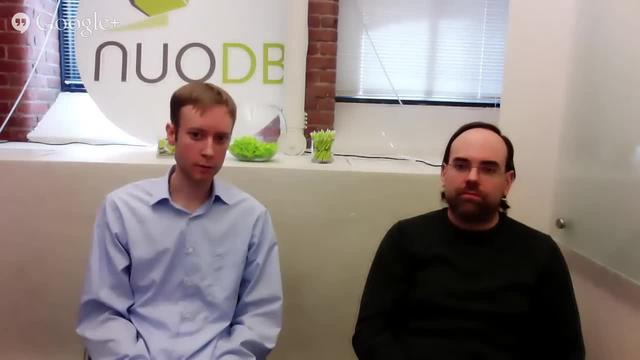 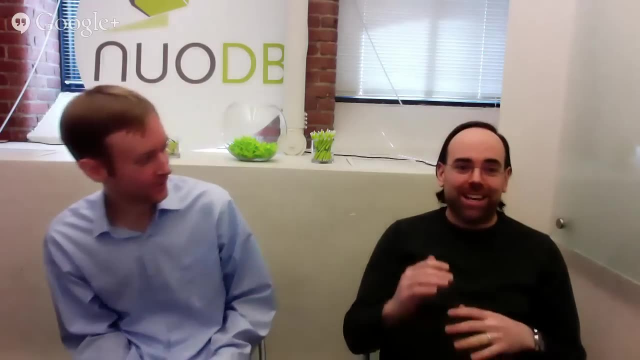 to latency spikes as they show up. Yeah, I think that optimism is important. It's really at the core of sort of the NuoDB philosophy. yeah, We're very optimistic here. you're saying We're like a glass half full kind of company. 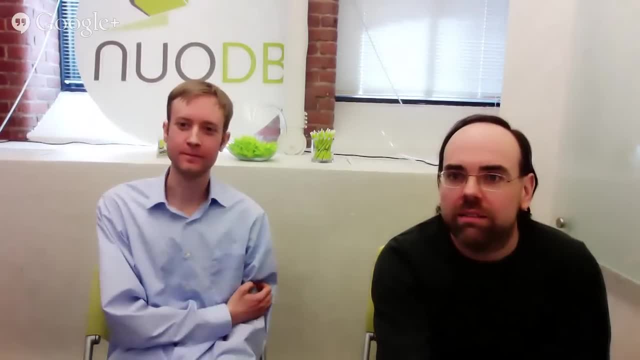 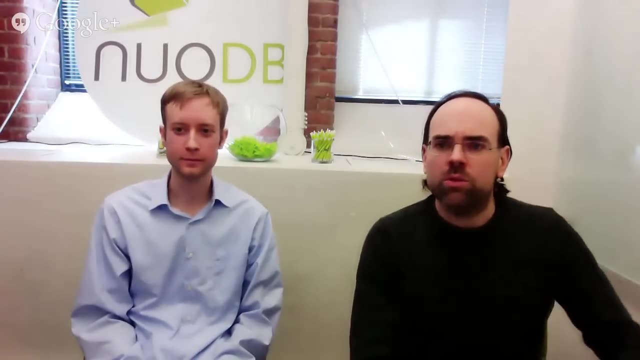 Yeah, All right, Cool. So let's see, I think I've been selecting. Oh, it's done, I see. Good, All right. Well, now I know how the interface works. So we got the question how NuoDB is innovative support for the cloud's dynamic. 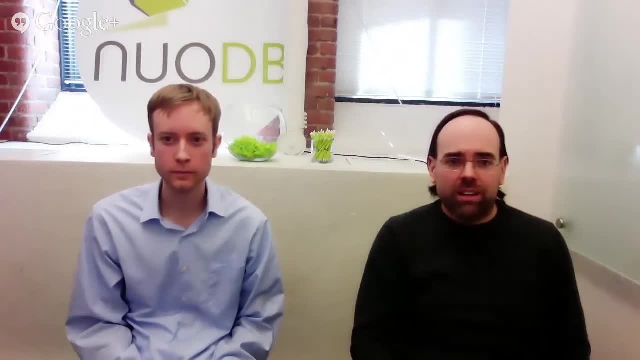 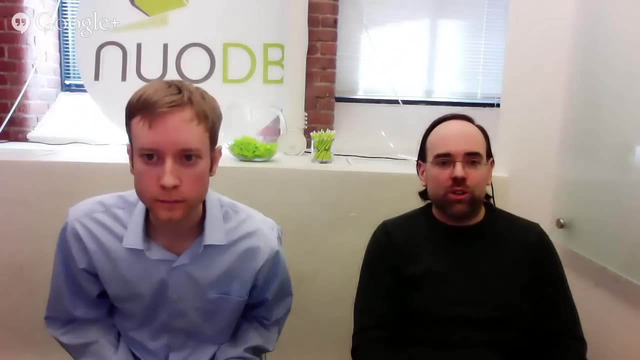 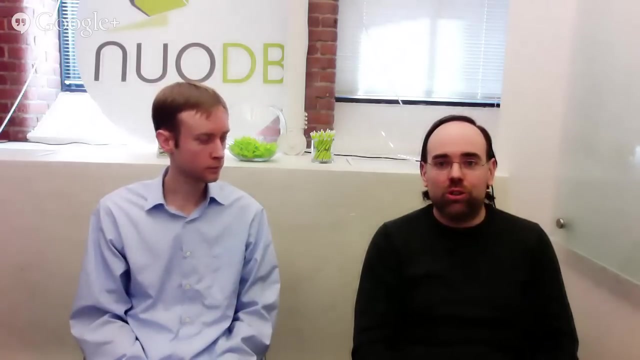 asynchronous nature and why is it called NuSQL? So I think that's the quick answer is: I think the NuSQL is really about people who are interested in solving kind of support for traditional SQL problems. right, You want SQL, you want assets, you want transactions, you want all the things that an RDBMS should. 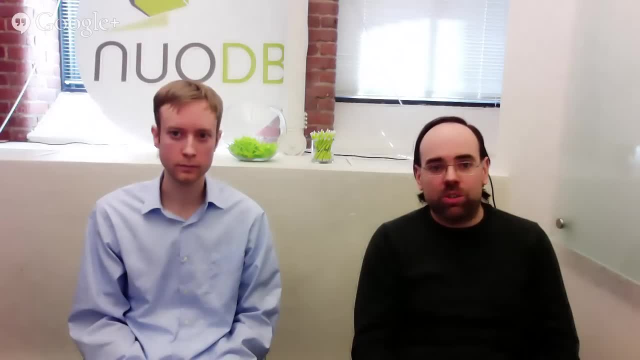 do. but you want to solve the kinds of new problems that traditional systems weren't designed for. So scale out kind of very agile, on demand, kind of the kinds of things you want in the cloud Security built in the ability to work across multiple data centers, the geo-distribution, 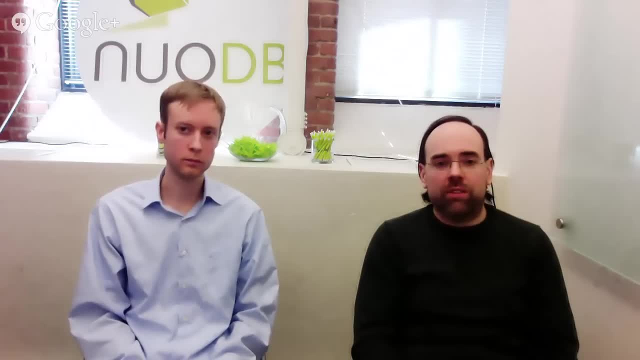 that Ross mentioned The elasticity Right- And that's where a lot of this comes from- right- Is that the outflow, Is that the algorithms that Ross is talking about are what we make into our core, because we assume that these kinds of systems are highly dynamic and we assume that things. 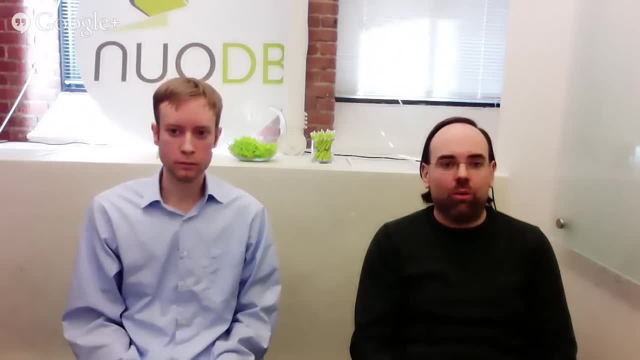 are constantly failing in distributed systems, that new processes are always coming online to take the place of things that failed. that you're doing upgrades, that you're moving between infrastructures. that you're picking one cloud one day and then going to a different. 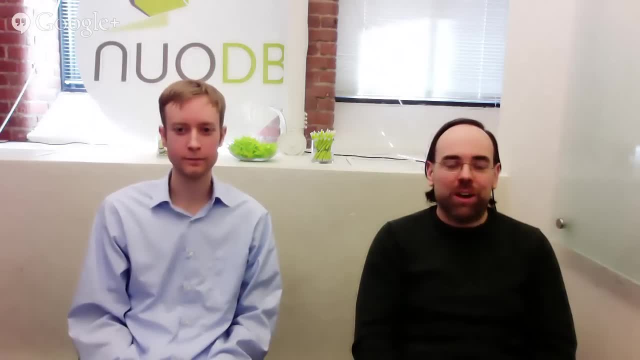 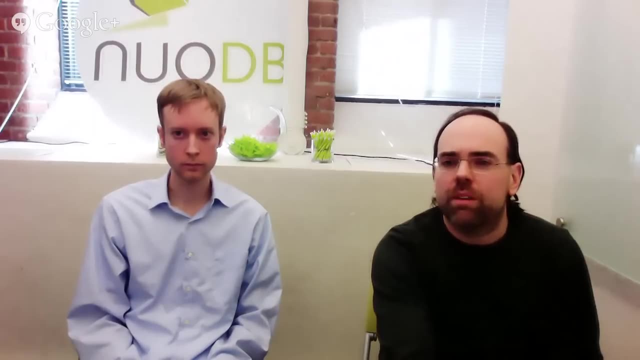 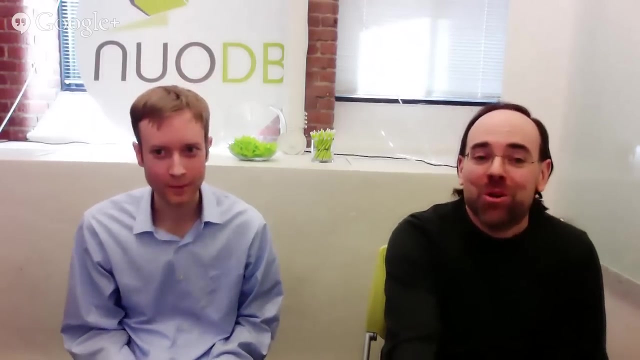 public cloud the next day, And so you have to be really kind of resilient and it's easy to kind of support those use cases. So I think that's really what we're talking about. Let's see. So this is probably a whole other webinar on its own. 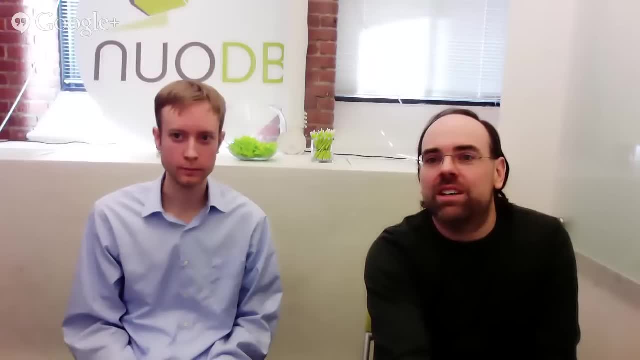 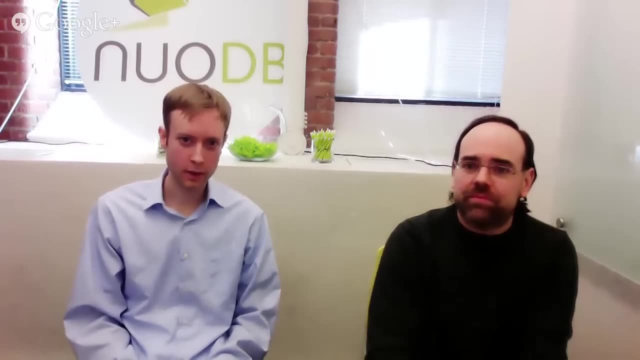 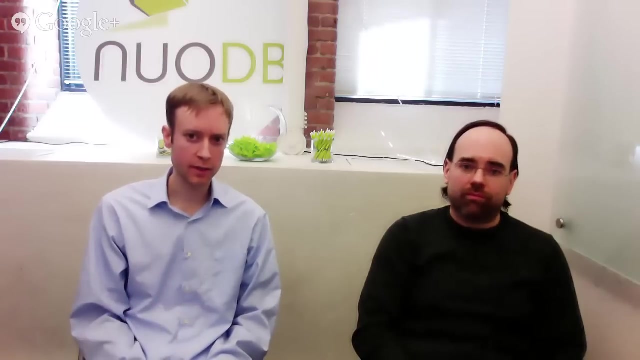 But, Ross, the question here from Luca is: how can you guarantee referential integrity in a distributed asynchronous database system? So referential integrity is not exactly my area of expertise, but I think that some of the topics that we've been talking about today can at least speak to those. 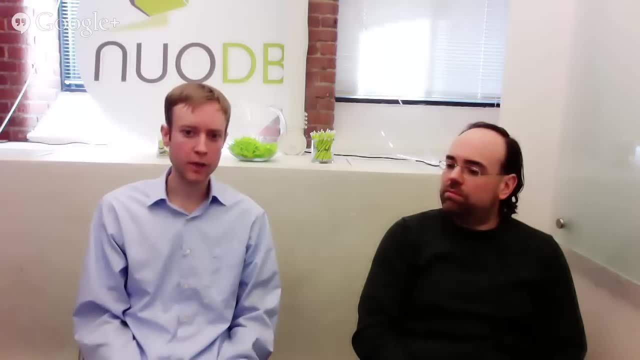 Okay. So let's get into this at a high level. You know when you – we have an asynchronous distributed system, but we also have means of coordinating those asynchronous tasks. So, when you have transactions which are executing asynchronously on multiple nodes and they 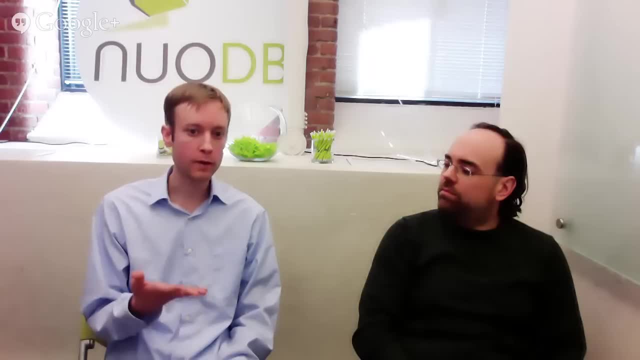 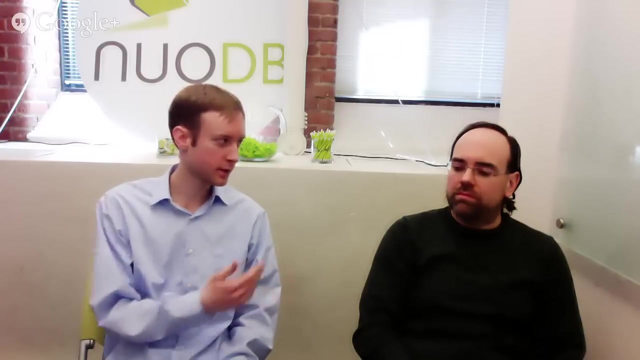 may be accessing at times the same atom. we resolve potential conflicts by coordinating via the chairman, And the chairman are chosen via this node list protocol, So that these low-level protocols, which Seth says are sort of baked into the core of the product, are at least at a low level how we guarantee things like referential integrity. 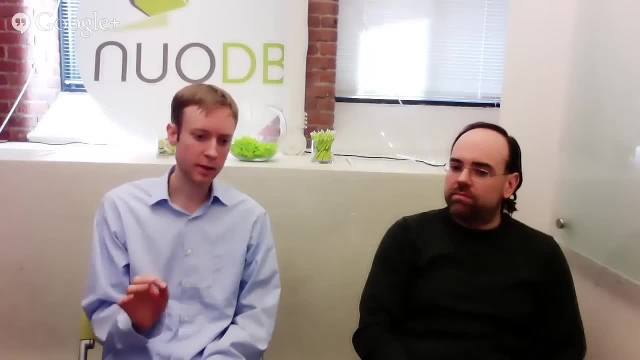 Now, of course, there's lots of protocols that are implemented sort of above this, what I think of as this sort of a storage layer, this atom layer, which kind of make referential integrity both possible and efficient, you know, things that are implemented by many. 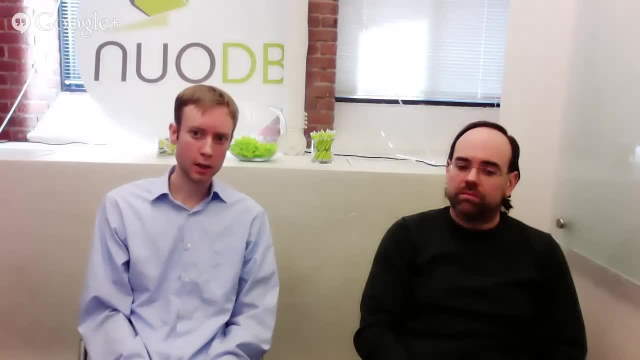 other engineers here make it efficient as well. and you know, maybe another unplugged session, we'll talk about those in more detail, but I think it's really the core protocols which make those possible, especially this idea of chairmanship or leadership, you know. 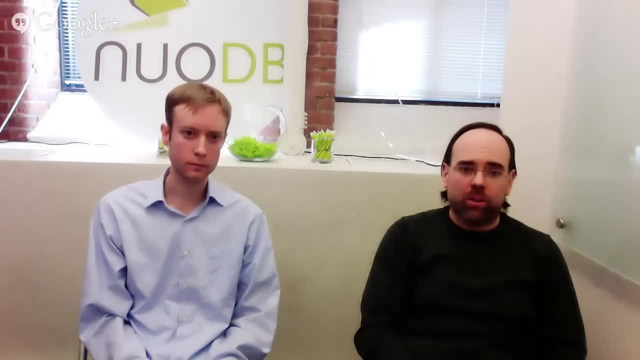 you really can't do it without that. Yeah and Luke, I definitely recommend you go check out our tech blog, because we talk in a lot more detail about kind of exactly what we're doing under the covers. I think this really gets to the core of what we're doing. 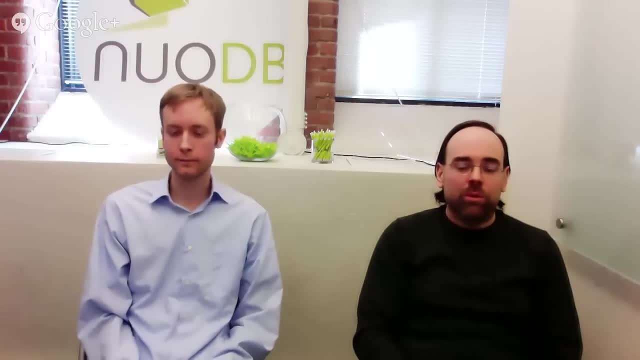 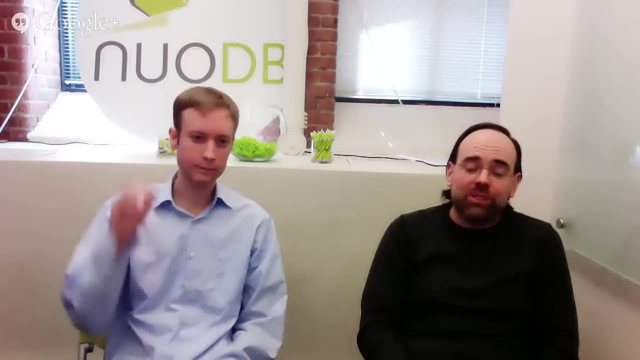 What we're doing differently here at NuoDB right, is we're really saying to solve these kinds of distributed referential integrity problems, you can't just kind of layer on top of an existing database and kind of put a little bit of replication in place. 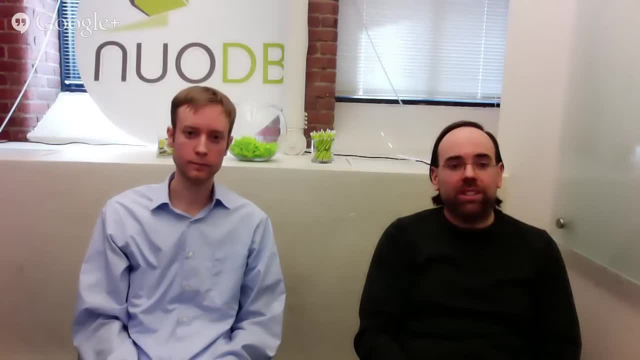 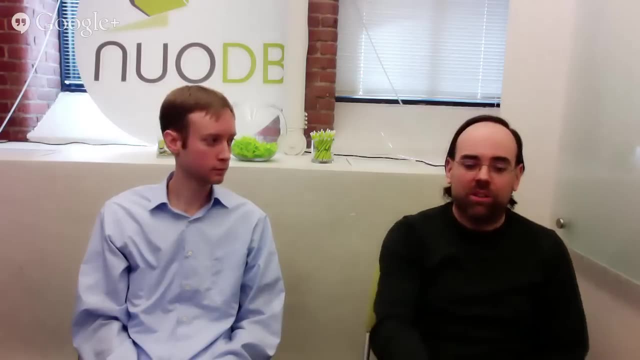 You really need to rethink the core protocols. you really need to rethink what the problems are you're trying to solve. you need to architect for the kinds of failures, the kinds of networks that Ross and I have been talking about so great, great question. 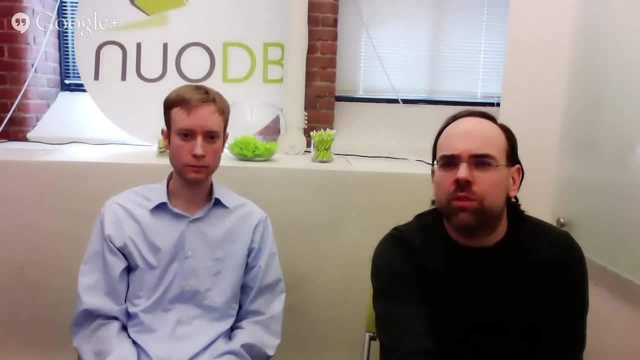 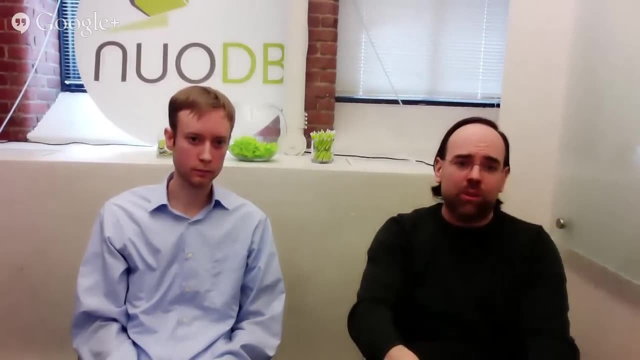 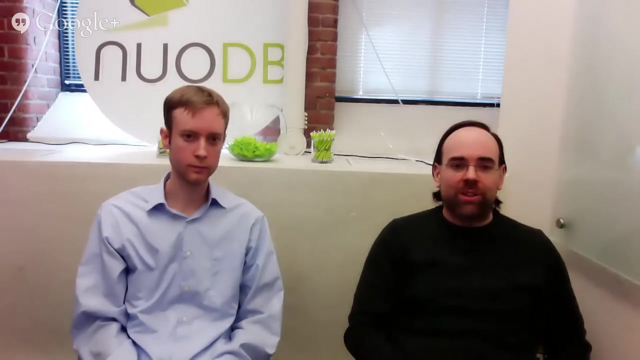 Let's see, We have a question from Riley that says: what are the steps you use to account for node failure? So, Riley, we're going to actually have a separate one of these sessions soon where we talk specifically about node failure. Node failure for us actually means a couple different things, because we think about kind. 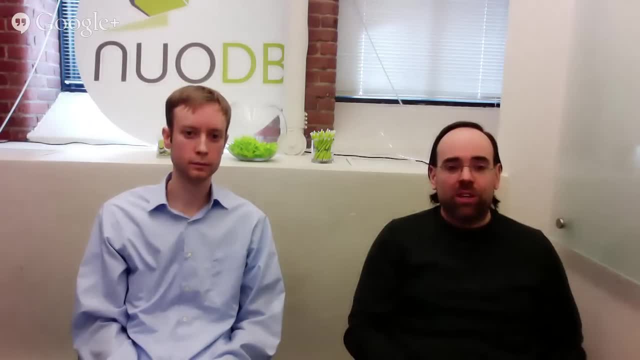 of processes in a database failing. We also think about potentially hosts failing in various ways, and this is a multi-tenant product. It can affect databases differently. that also affects our management here. and then, of course, when you're thinking about widely distributed systems, you get even more interesting. 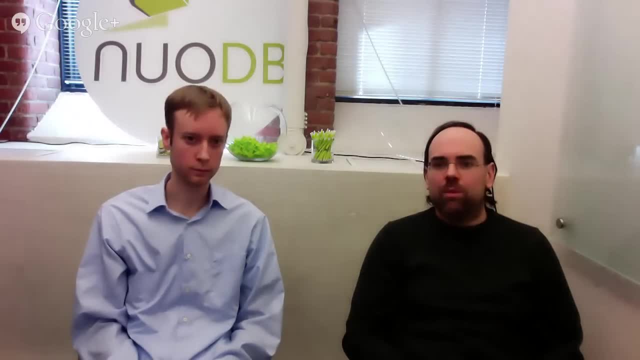 failures around networks and everything else. But, Ross, I think you kind of talked a little bit about this in the sense that one of these steps that's really important is understanding something about when you are facing failure, knowing something about where the authorities are for something. 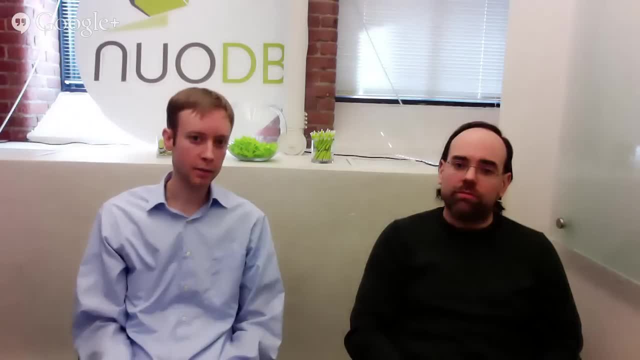 Can I? Yeah, So the basic idea behind node failure is that you have to know where the authorities are right, And that's kind of what we're trying to do with Node Failure is. I think that, basically, what we do is fairly standard. We have some tricks sort of baked into the product which I think are unique but sort of the core ideas are fairly easy to understand. We have things like heartbeats which are going out to see whether nodes are still alive. We're keeping the node list again up to date to see who's actually still caching atoms.